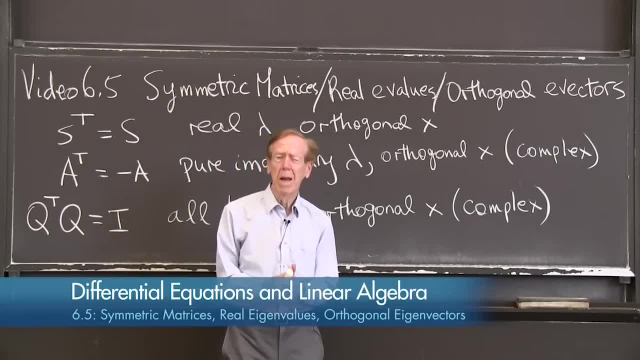 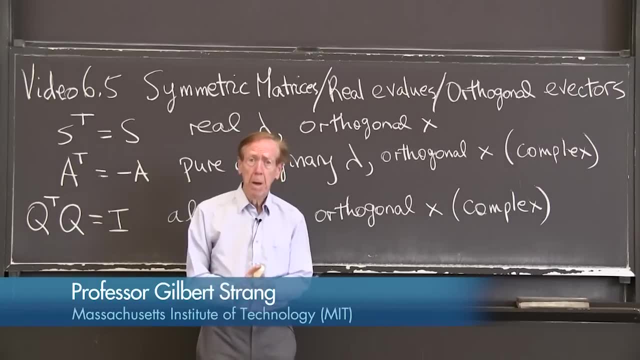 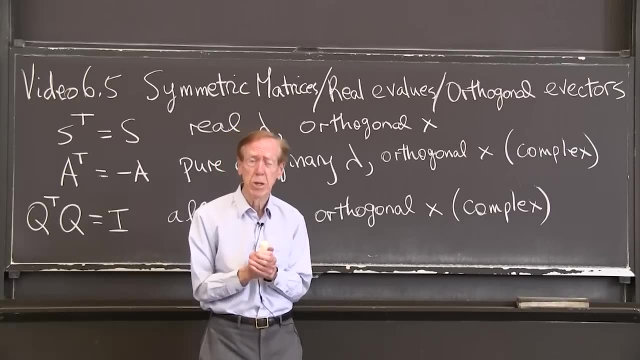 OK, So this is a prepare the way video about symmetric matrices and complex matrices. We'll see symmetric matrices in second order systems of differential equations. Symmetric matrices are the best. They have special properties and we want to see what are the special properties of the eigenvalues. 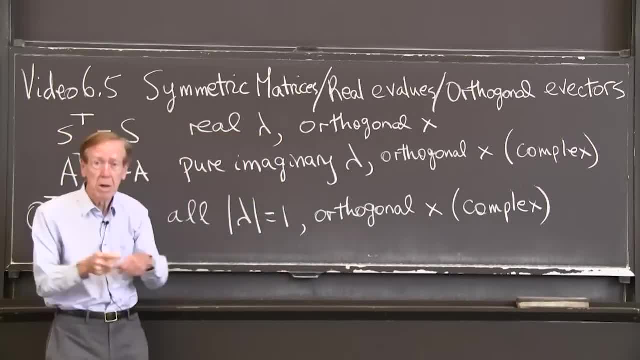 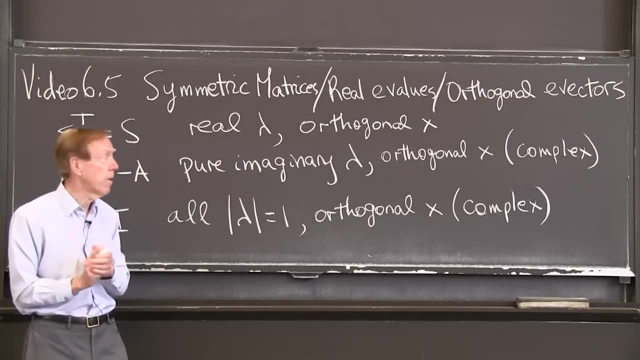 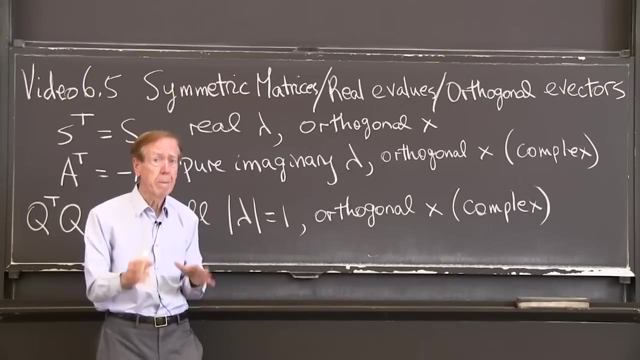 and the eigenvectors, And I guess the title of this lecture tells you what those properties are. So if a matrix is symmetric- and I'll use capital S for symmetric matrix- the first point is the eigenvalues are real, which is not automatic. 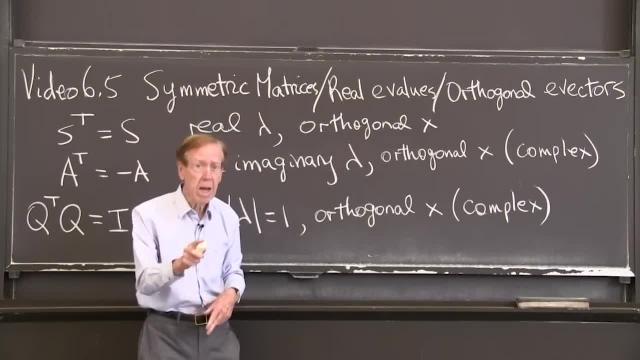 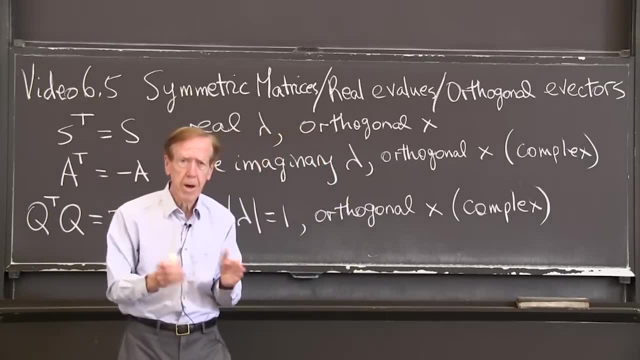 But it's always true if the matrix is symmetric. And the second, even more special point is that the eigenvectors are perpendicular to each other. Different eigenvectors for different eigenvalues come out, Not perpendicular. Those are beautiful properties. 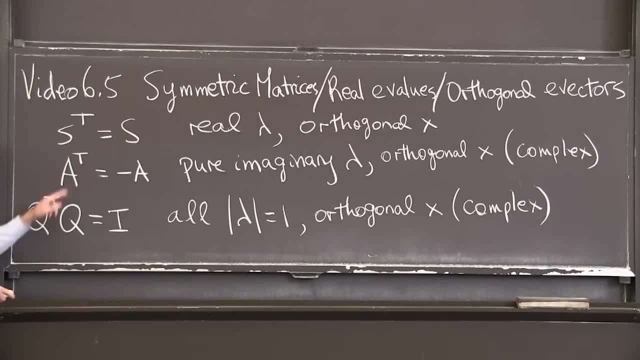 They pay off. So can I actually? so that's the symmetric matrix and that's what I just said. Real lambda orthogonal x. Also, we could look at anti-symmetric matrices. The transpose is minus the matrix. In that case we don't have real eigenvalues. 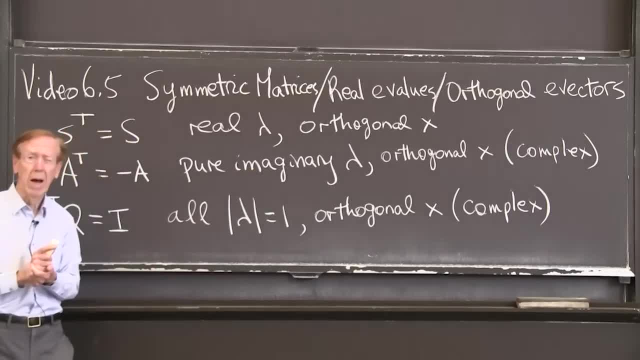 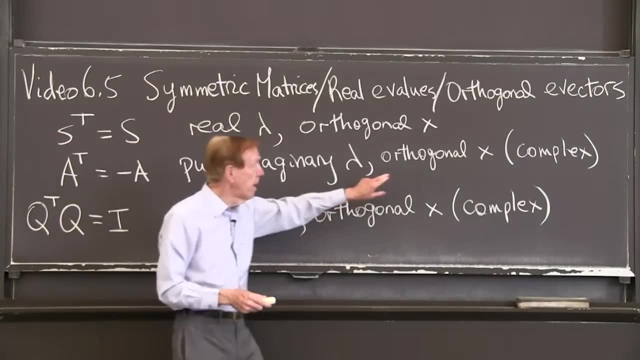 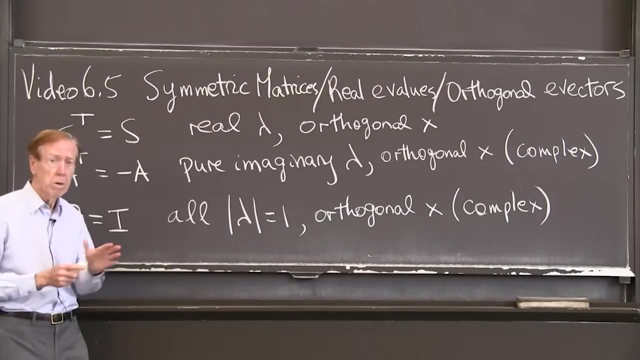 In fact, we are sure to have pure imaginary eigenvalues. i times something, Something On the imaginary axis, But again the eigenvectors will be orthogonal. However, they will also be complex When we have anti-symmetric matrices. 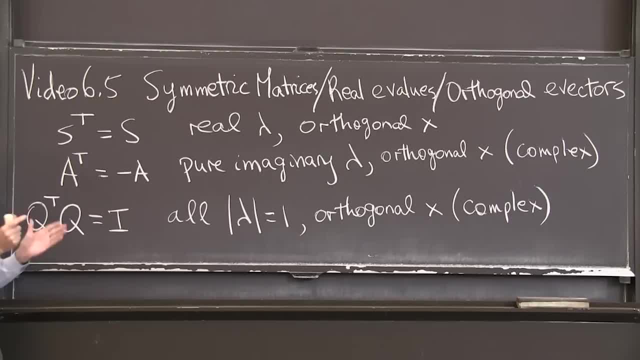 we get into complex numbers Can't help it, Even if the matrix is real. And then, finally, is the family of orthogonal matrices, And those matrices have eigenvalues of size 1. Possibly complex, But the magnitude of the number is 1.. 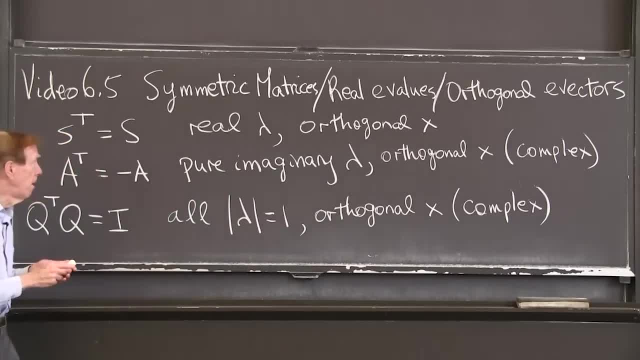 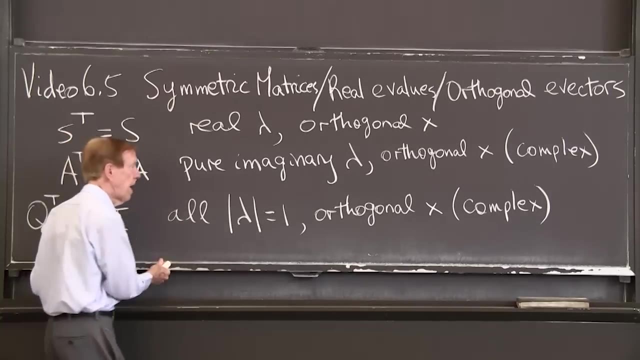 And again, the eigenvectors are orthogonal. This is the great family of real, imaginary and unit circle for the eigenvalues. OK, I want to do examples, So I'll just have an example of every one. So there's a symmetric matrix. 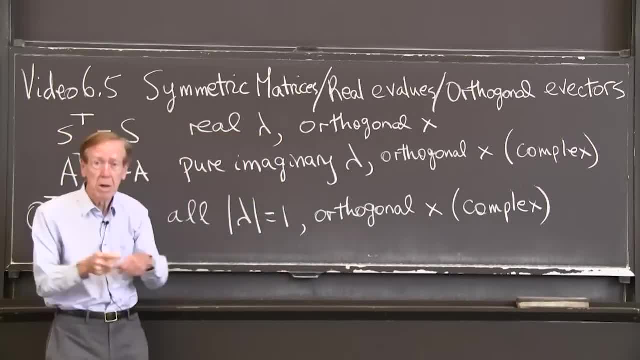 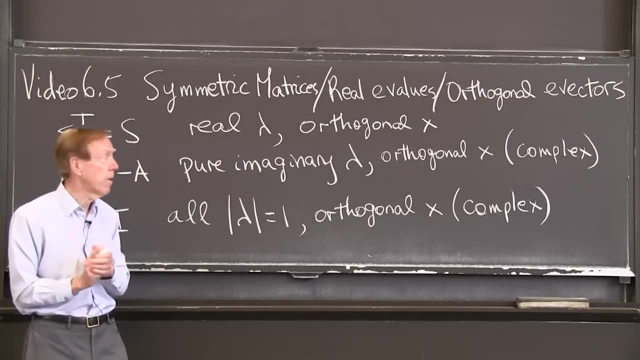 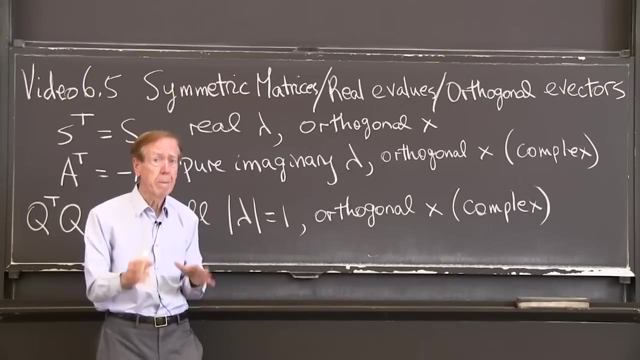 and the eigenvectors, And I guess the title of this lecture tells you what those properties are. So if a matrix is symmetric- and I'll use capital S for symmetric matrix- the first point is the eigenvalues are real, which is not automatic. 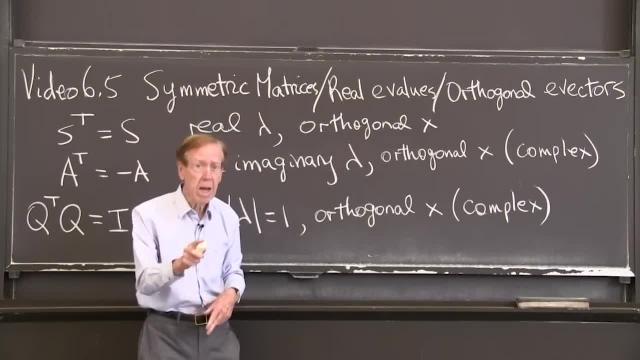 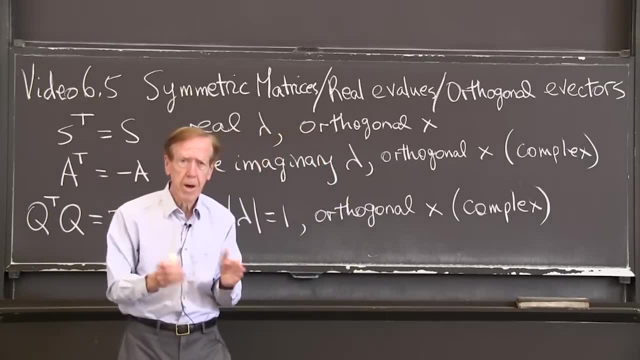 But it's always true if the matrix is symmetric. And the second, even more special point is that the eigenvectors are perpendicular to each other. Different eigenvectors for different eigenvalues come out, Not perpendicular. Those are beautiful properties. 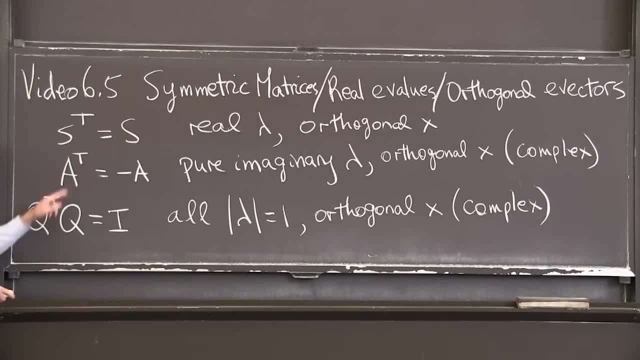 They pay off. So can I actually? so that's the symmetric matrix and that's what I just said. Real lambda orthogonal x. Also, we could look at anti-symmetric matrices. The transpose is minus the matrix. In that case we don't have real eigenvalues. 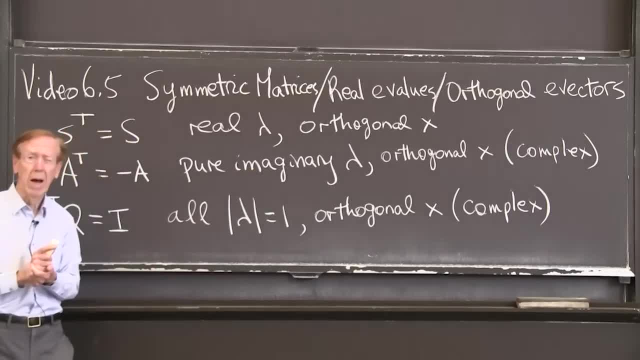 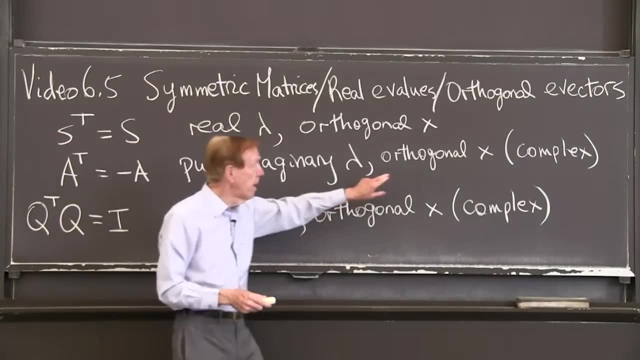 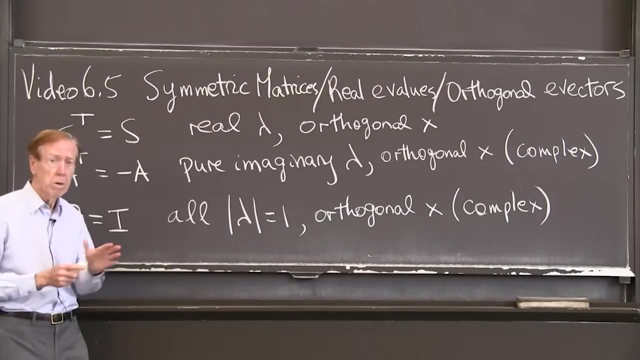 In fact, we are sure to have pure imaginary eigenvalues. i times something, Something On the imaginary axis, But again the eigenvectors will be orthogonal. However, they will also be complex When we have anti-symmetric matrices. 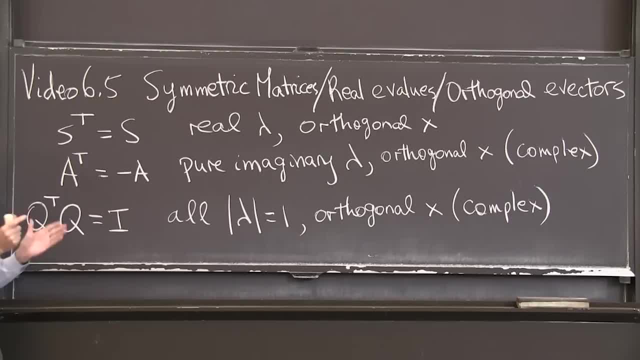 we get into complex numbers Can't help it, Even if the matrix is real. And then, finally, is the family of orthogonal matrices, And those matrices have eigenvalues of size 1. Possibly complex, But the magnitude of the number is 1.. 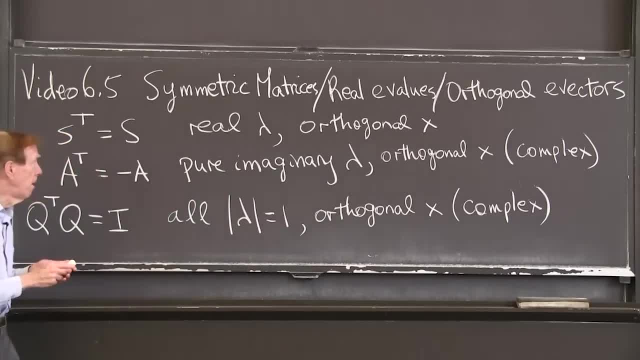 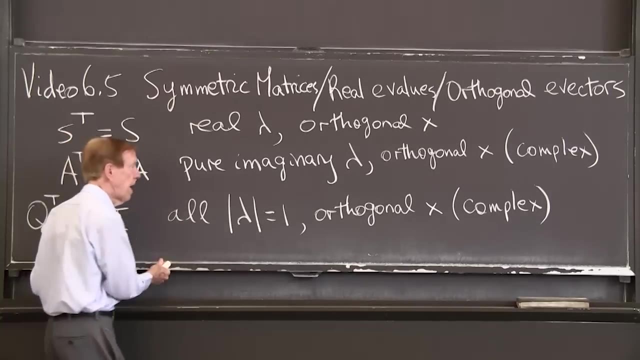 And again, the eigenvectors are orthogonal. This is the great family of real, imaginary and unit circle for the eigenvalues. OK, I want to do examples, So I'll just have an example of every one. So there's a symmetric matrix. 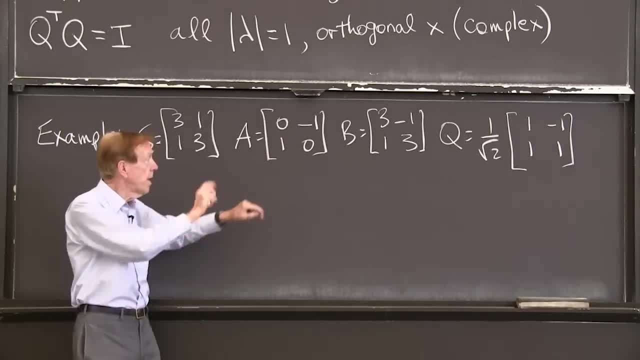 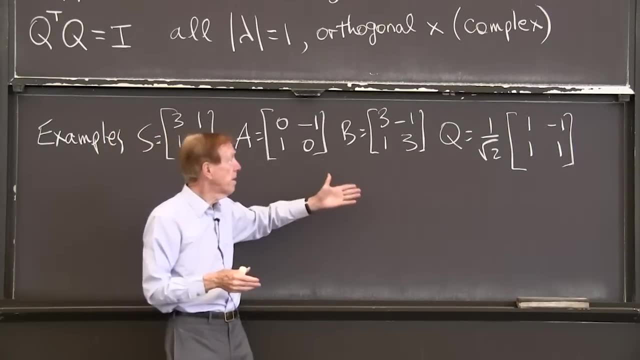 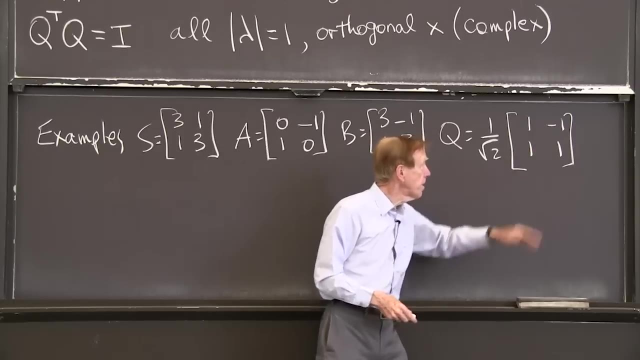 There's an anti-symmetric matrix. If I transpose it it changes sign. Here is a combination- Not symmetric, not anti-symmetric, but still a good matrix. And there is an orthogonal matrix, orthogonal columns, And those columns have length 1.. 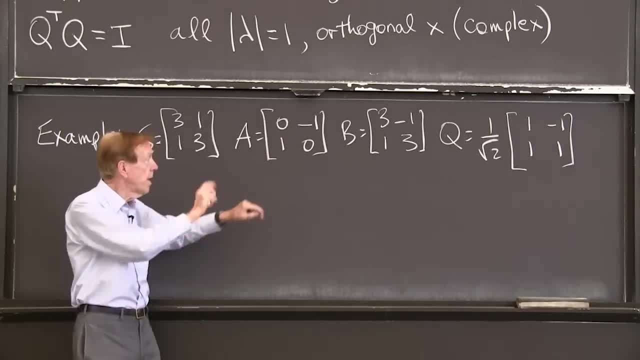 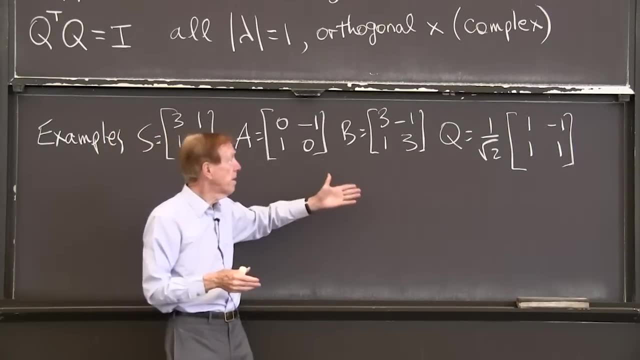 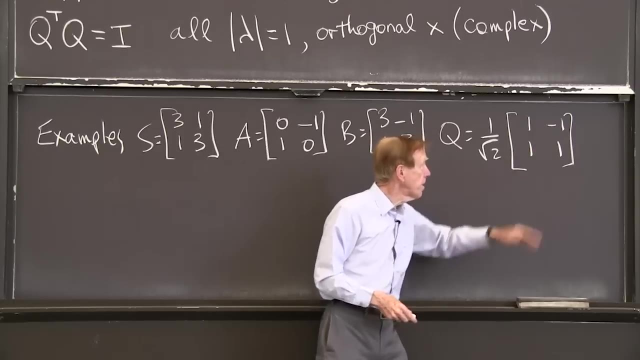 There's an anti-symmetric matrix. If I transpose it it changes sign. Here is a combination- Not symmetric, not anti-symmetric, but still a good matrix. And there is an orthogonal matrix, orthogonal columns, And those columns have length 1.. 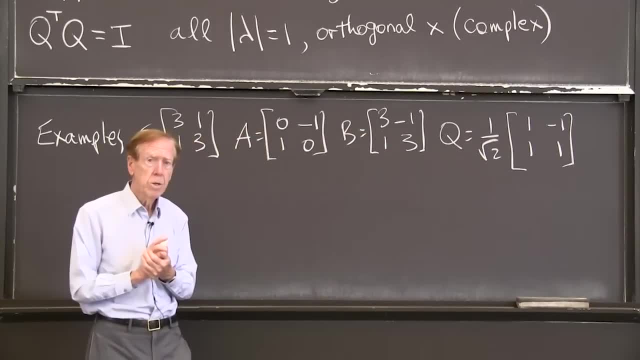 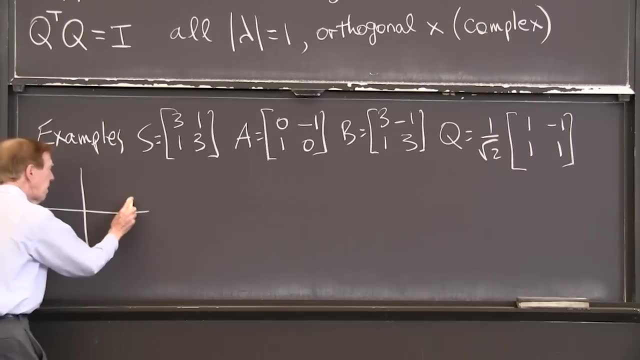 That's why I've got the square root of 2 in there. So these are the special matrices here You could say. can I just draw a little picture of the complex plane? There is the real axis, Here is the imaginary axis. 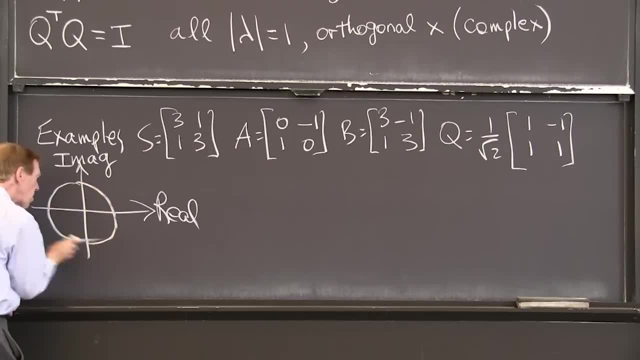 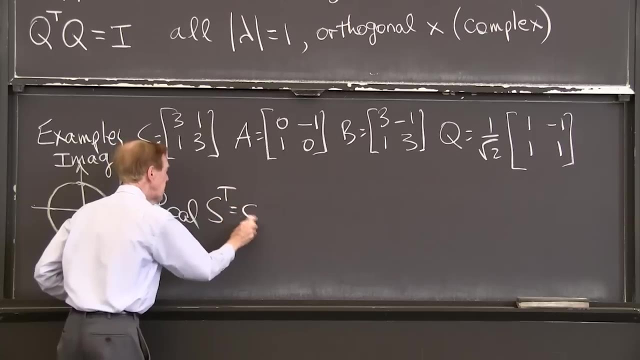 And here's the unit circle, Not greatly circular, but close Now. so this is real. Eigenvalues are on the real axis. When the real axis is on the imaginary axis, it's not circular. It's not circular, They're on the imaginary axis. when s transpose equals s, 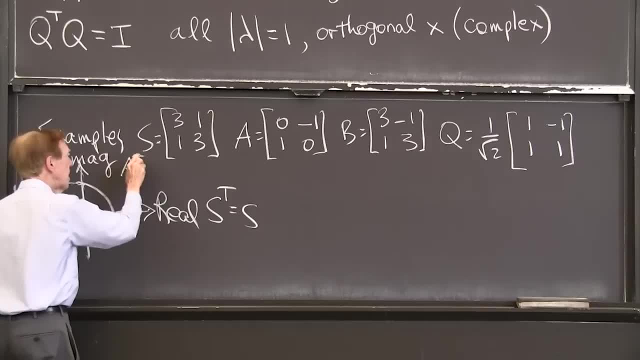 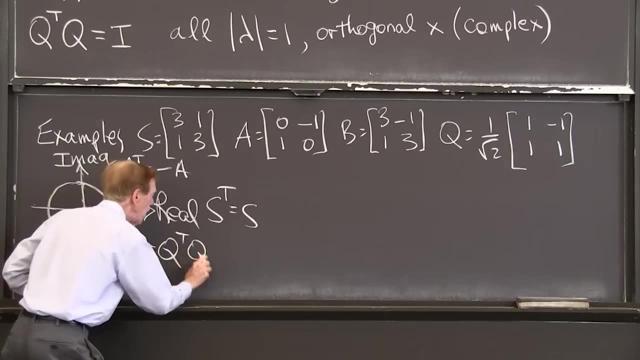 They're on the imaginary axis when a transpose equals minus a And they're on the unit circle when q transpose q is the identity. q transpose is q inverse. in this case, q transpose is q inverse. Here the transpose is the matrix. Here the transpose is minus the matrix. 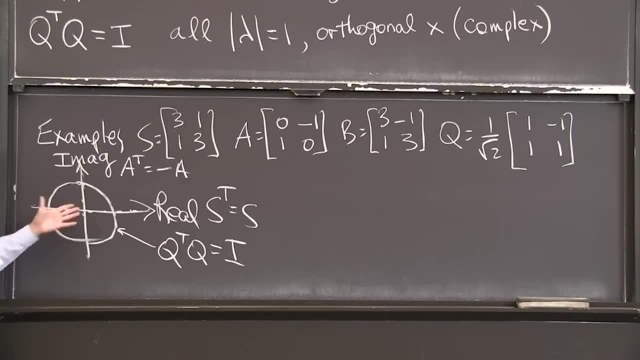 And you see the beautiful picture of eigenvalues where they are, And the eigenvectors for all of those are orthogonal. Let me find them Here. that symmetric matrix has lambda as 2 and 4.. The trace is 6.. The determinant is 8.. 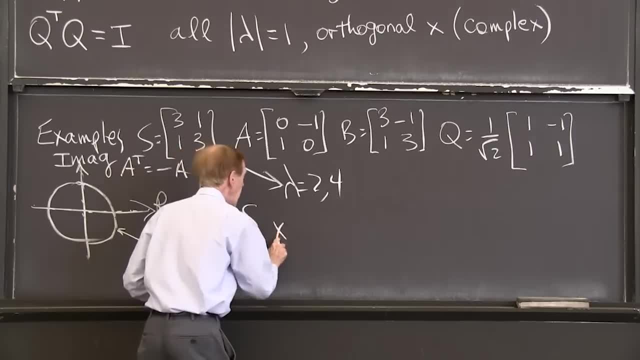 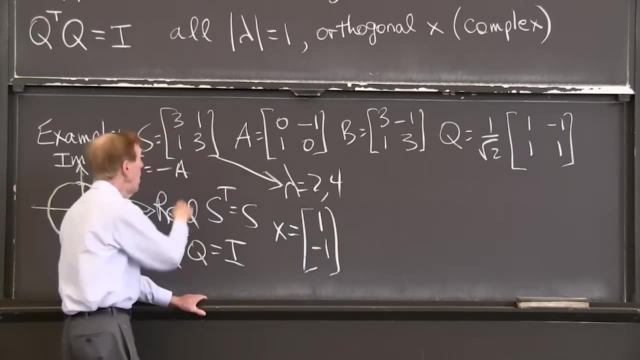 That's the right answer. Lambda equal 2 and 4.. And x would be 1 and minus 1 for 2. And for 4, it's 1 and 1.. Orthogonal, Orthogonal eigenvectors. Take the dot product of those. 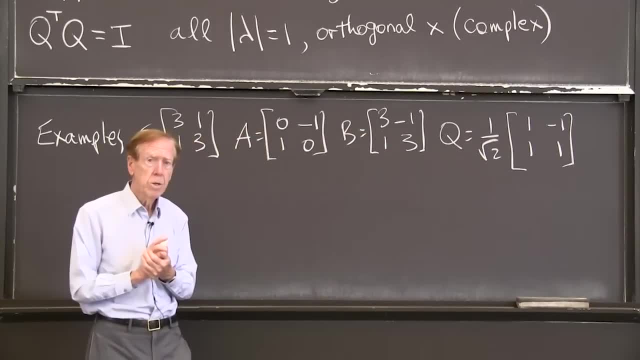 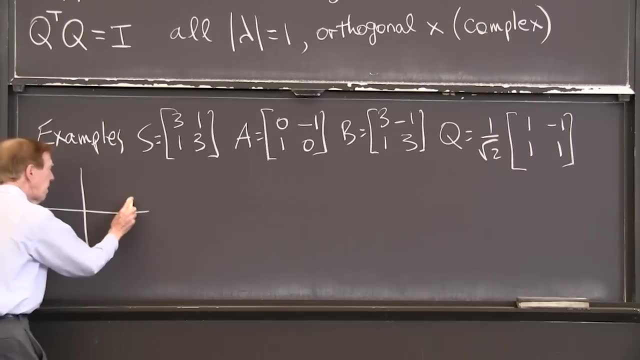 That's why I've got the square root of 2 in there. So these are the special matrices here You could say. can I just draw a little picture of the complex plane? There is the real axis, Here is the imaginary axis. 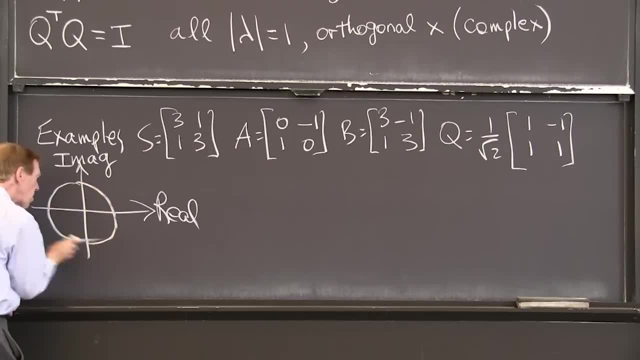 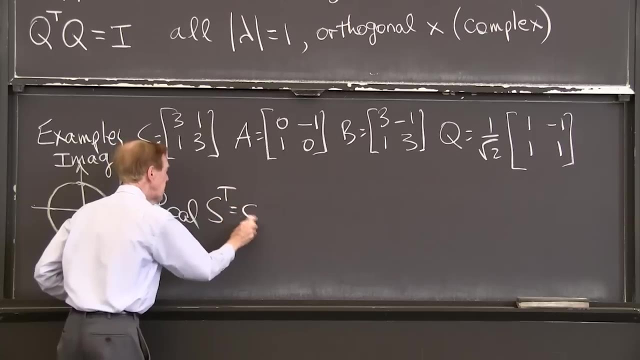 And here's the unit circle, Not greatly circular, but close Now. so this is real. Eigenvalues are on the real axis. When the real axis is on the imaginary axis, it's not circular. It's not circular, They're on the imaginary axis. when s transpose equals s, 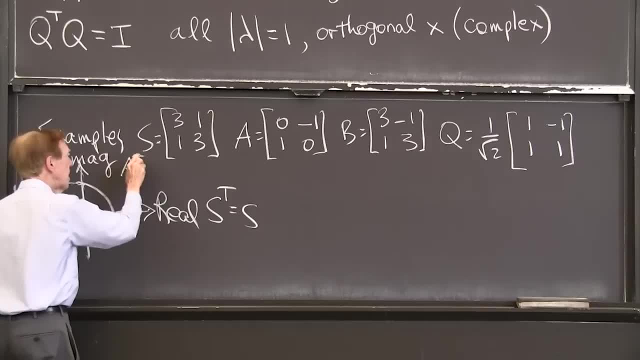 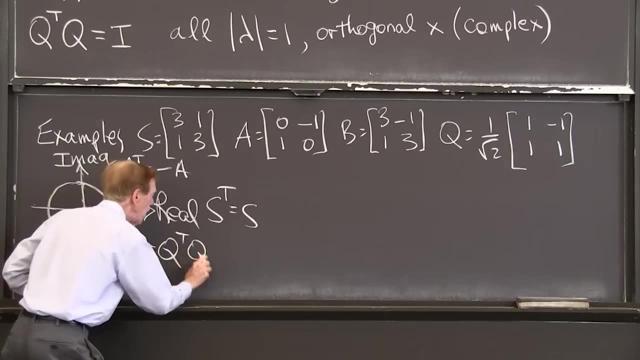 They're on the imaginary axis when a transpose equals minus a And they're on the unit circle when q transpose q is the identity. q transpose is q inverse. in this case, q transpose is q inverse. Here the transpose is the matrix. Here the transpose is minus the matrix. 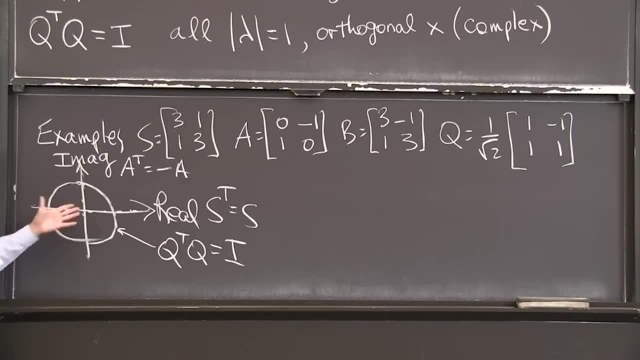 And you see the beautiful picture of eigenvalues where they are, And the eigenvectors for all of those are orthogonal. Let me find them Here. that symmetric matrix has lambda as 2 and 4.. The trace is 6.. The determinant is 8.. 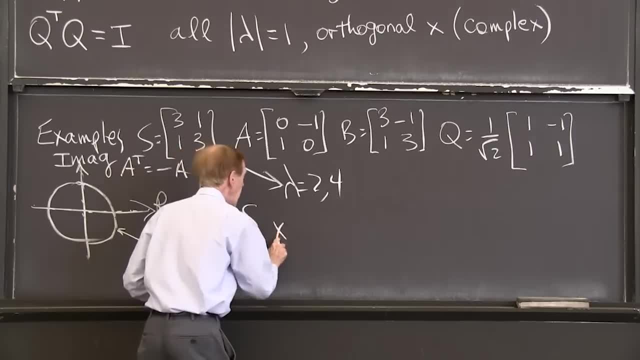 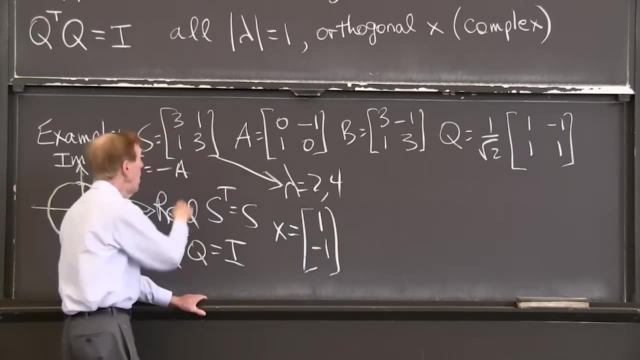 That's the right answer. Lambda equal 2 and 4.. And x would be 1 and minus 1 for 2. And for 4, it's 1 and 1.. Orthogonal, Orthogonal eigenvectors. Take the dot product of those. 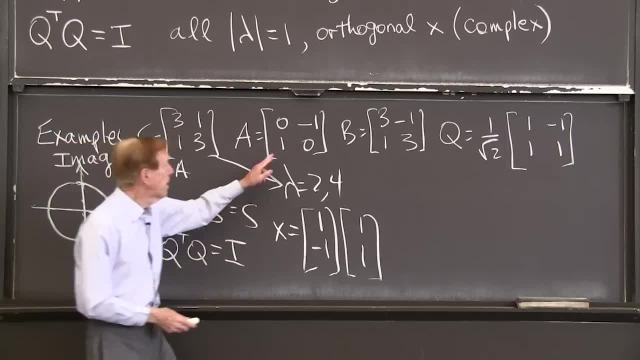 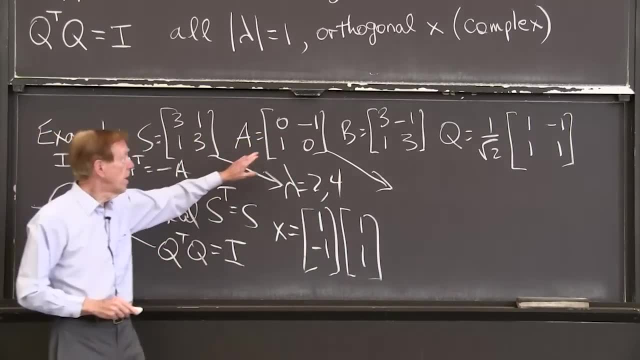 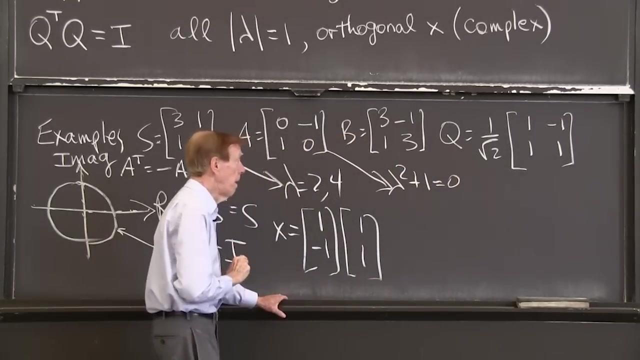 You get 0.. And real eigenvalues. What about a Antisymmetric? The equation? when I do determinant of lambda minus a, I get lambda squared Plus 1 equals 0. for this one, That leads me to lambda squared plus 1 equals 0.. 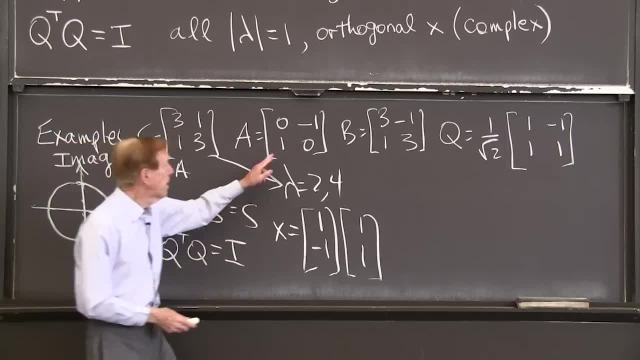 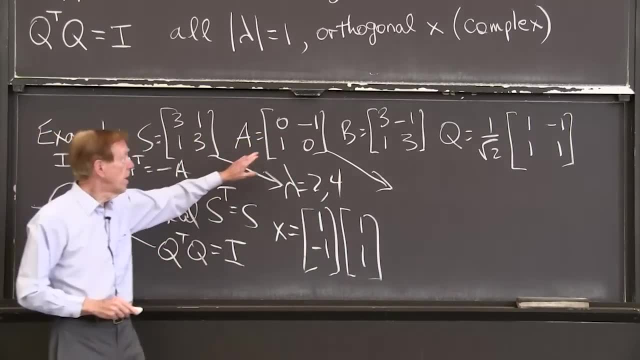 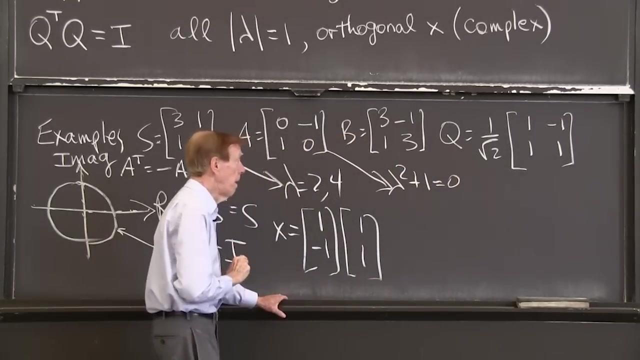 You get 0.. And real eigenvalues. What about a Antisymmetric? The equation? when I do determinant of lambda minus a, I get lambda squared Plus 1 equals 0. for this one, That leads me to lambda squared plus 1 equals 0.. 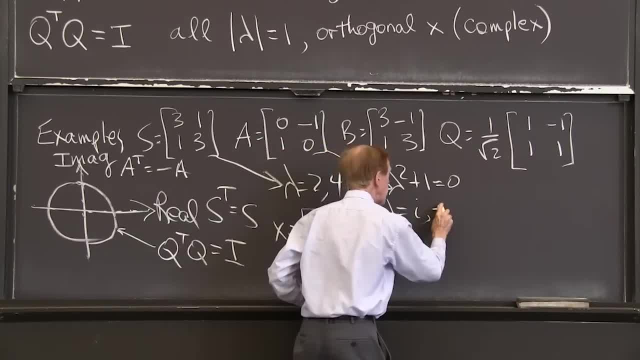 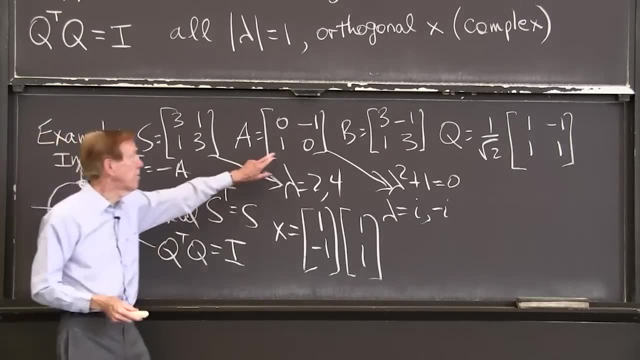 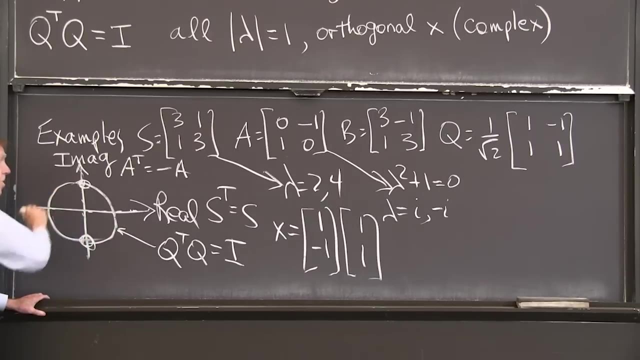 So that gives me lambda is i and minus i, as promised, on the imaginary axis, And I guess that that matrix is also an orthogonal matrix And those eigenvalues i and minus i are also on the circle, So that a is also a q. 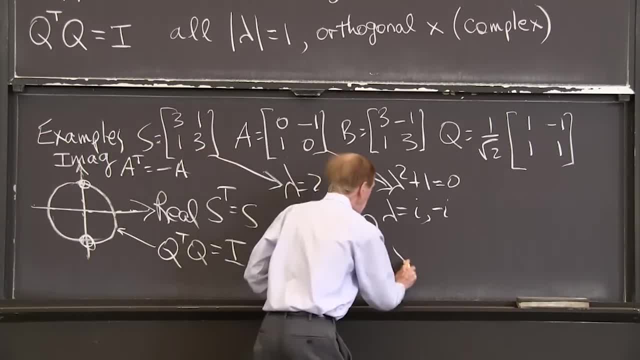 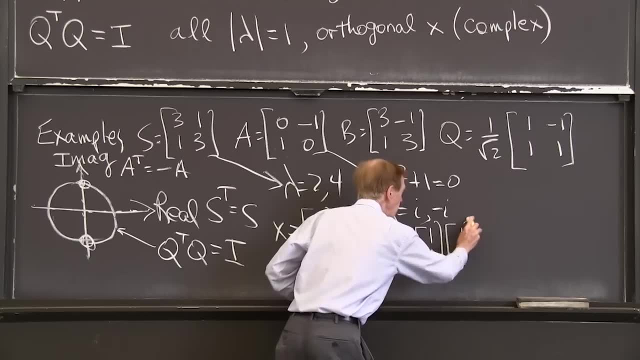 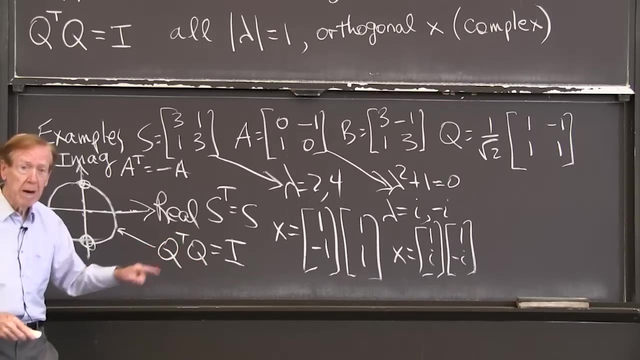 OK, What are the eigenvectors for that? I think that the eigenvectors turn out to be 1i and 1 minus i. Oh, those are orthogonal. I'll have to tell you about orthogonality for complex vectors. 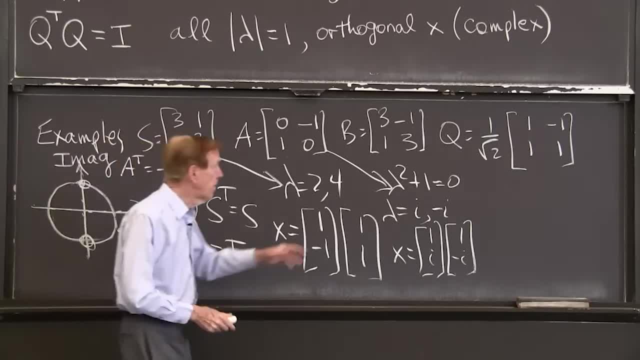 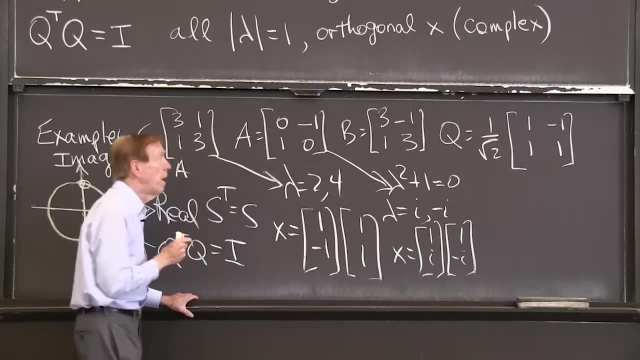 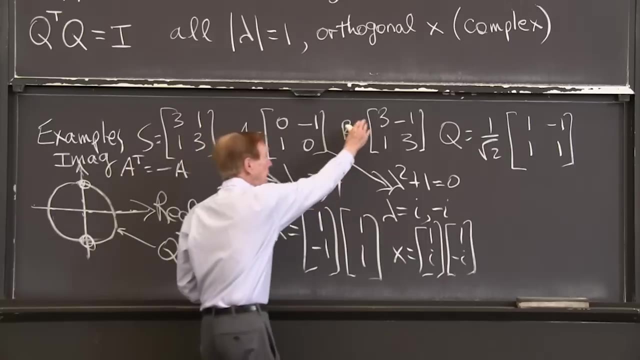 Let me complete these examples. What about the eigenvalues of this one? Well, that's an easy one. Can you connect that to a? This is just b, is just a plus 3 times the identity? to put 3's on the diagonal. 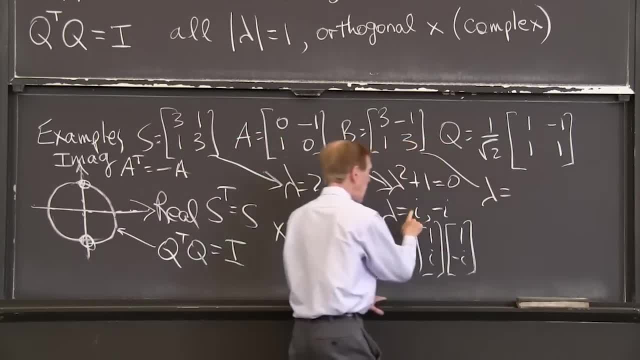 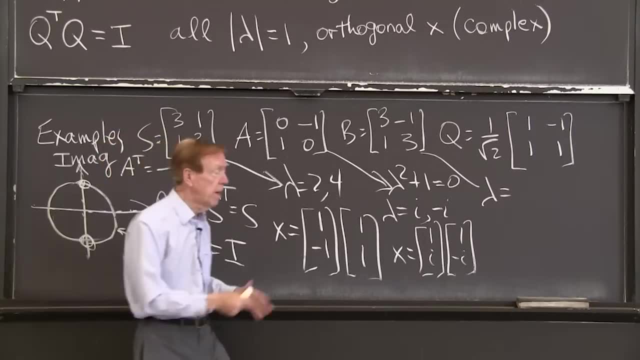 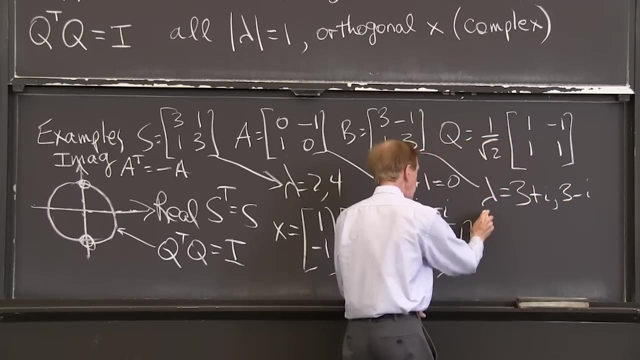 So I'm expecting- here the lambdas are, if here they were- i and minus i. all I've done is add 3 times the identity, So I'm just adding 3.. I'm shifting by 3.. I'll have 3 plus i and 3 minus i and the same eigenvectors. 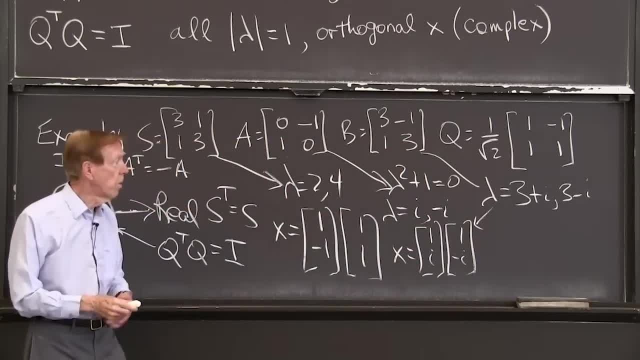 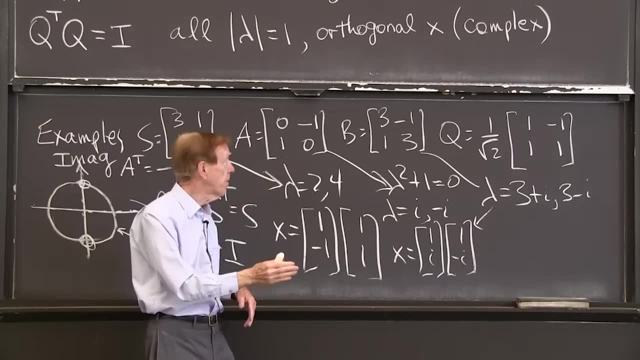 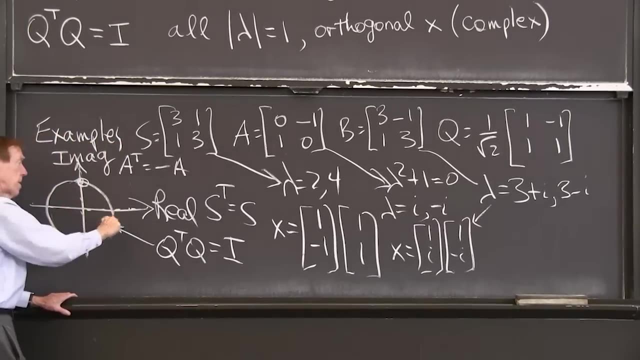 And now, so that's a complex number. That matrix was not perfectly anti-symmetric, It's not perfectly symmetric. So that gave me a 3 plus i somewhere, not on the axis or that axis or the circle Out there- 3 plus i and 3 minus i. 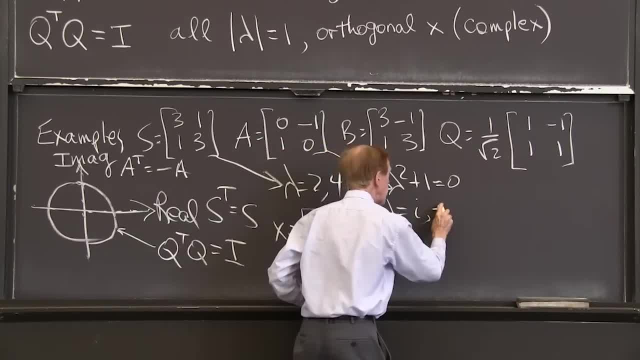 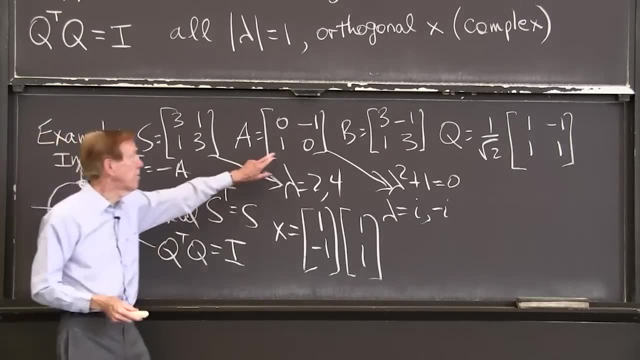 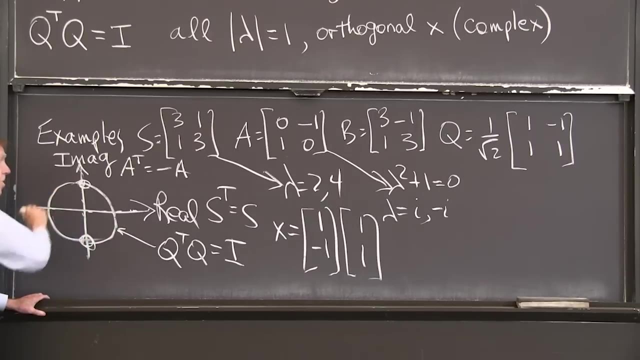 So that gives me lambda is i and minus i, as promised, on the imaginary axis, And I guess that that matrix is also an orthogonal matrix And those eigenvalues i and minus i are also on the circle, So that a is also a q. 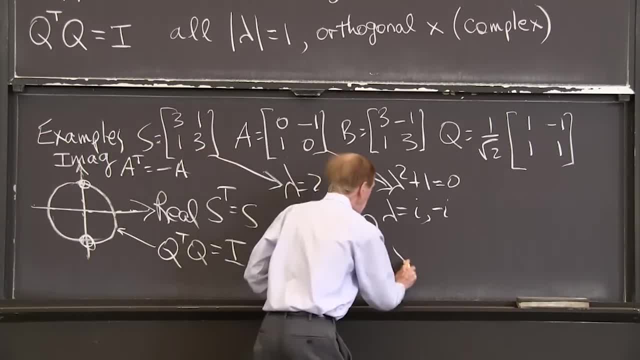 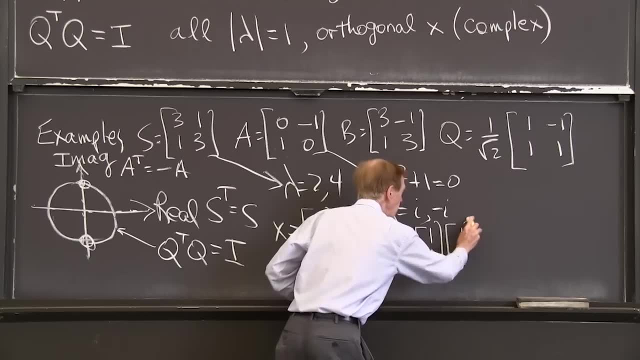 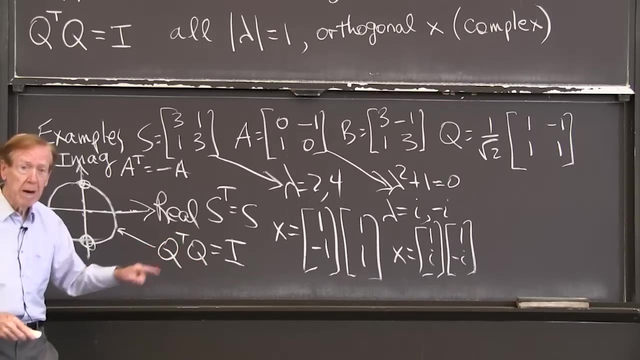 OK, What are the eigenvectors for that? I think that the eigenvectors turn out to be 1i and 1 minus i. Oh, those are orthogonal. I'll have to tell you about orthogonality for complex vectors. 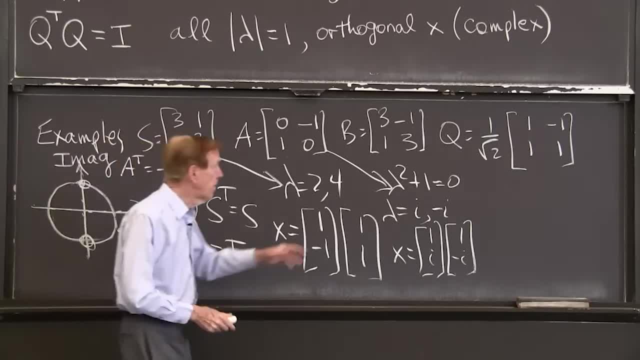 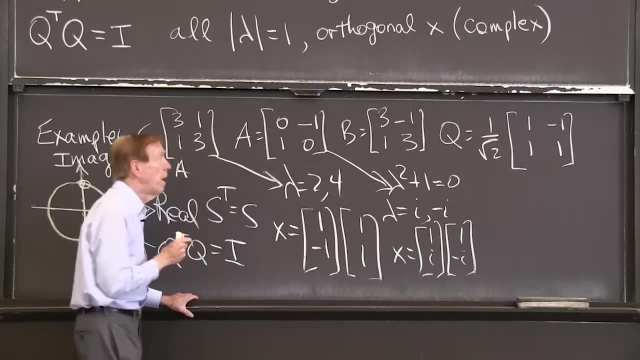 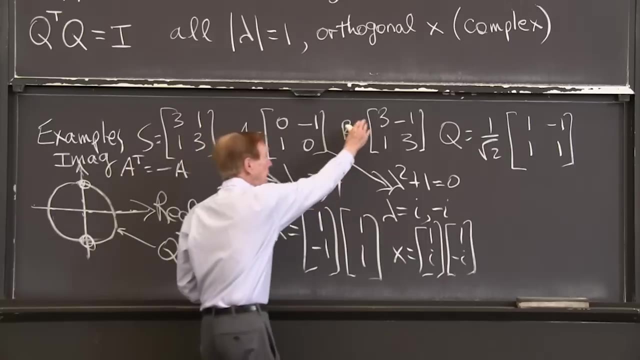 Let me complete these examples. What about the eigenvalues of this one? Well, that's an easy one. Can you connect that to a? This is just b, is just a plus 3 times the identity? to put 3's on the diagonal. 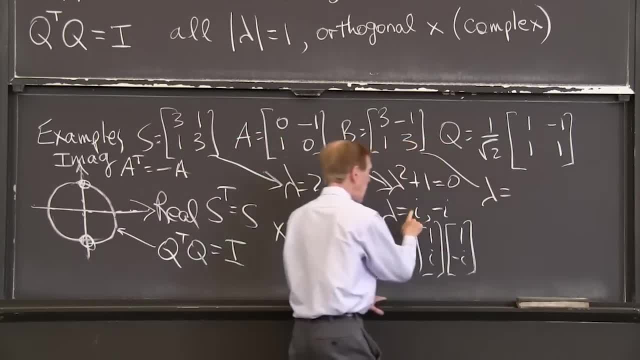 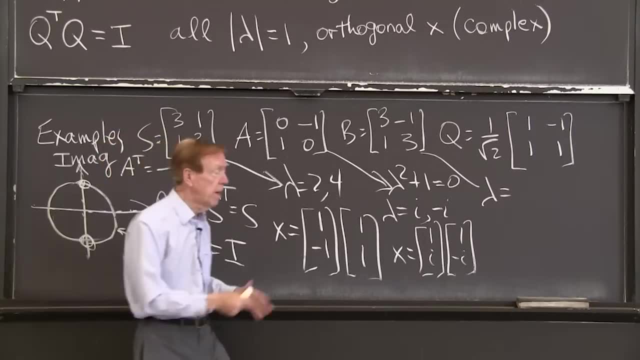 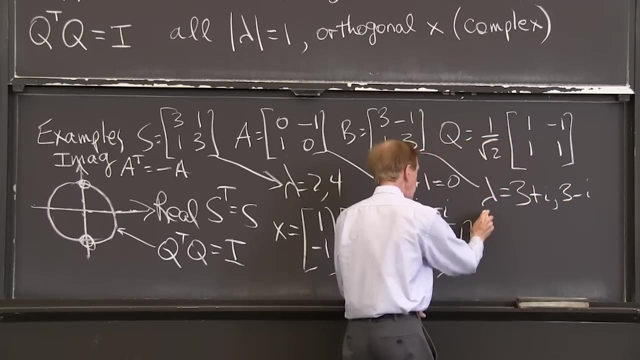 So I'm expecting- here the lambdas are, if here they were- i and minus i. all I've done is add 3 times the identity, So I'm just adding 3.. I'm shifting by 3.. I'll have 3 plus i and 3 minus i and the same eigenvectors. 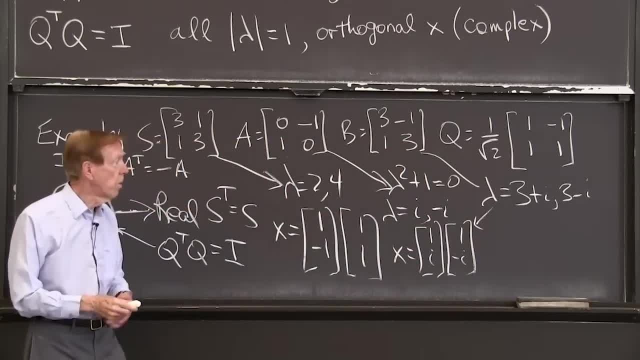 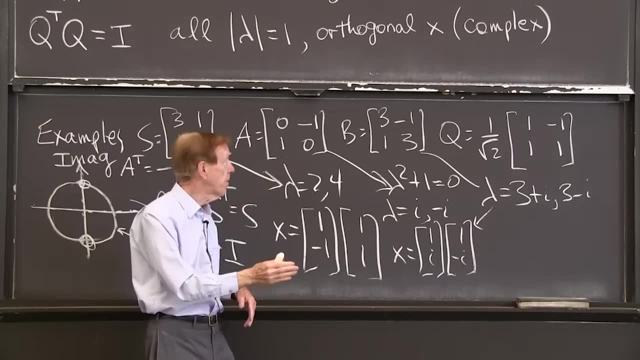 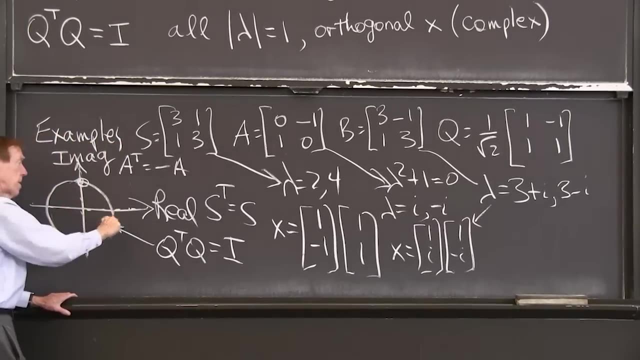 And now, so that's a complex number. That matrix was not perfectly anti-symmetric, It's not perfectly symmetric. So that gave me a 3 plus i somewhere, not on the axis or that axis or the circle Out there- 3 plus i and 3 minus i. 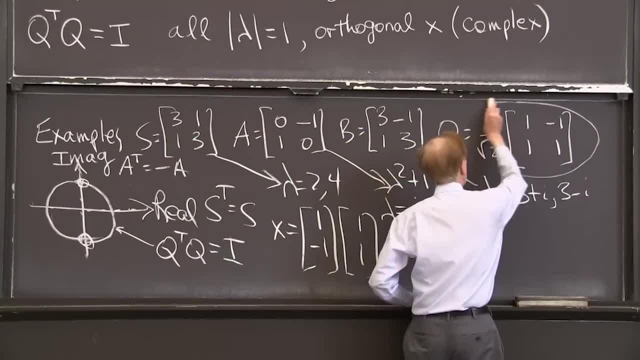 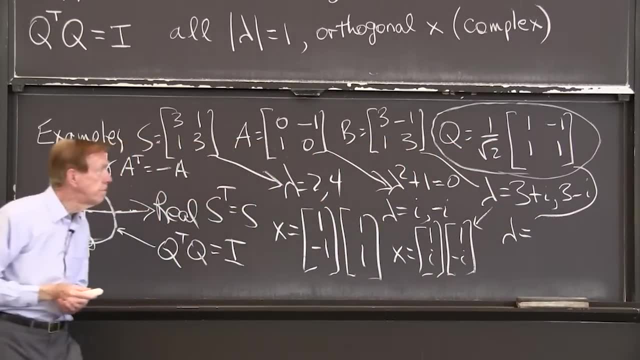 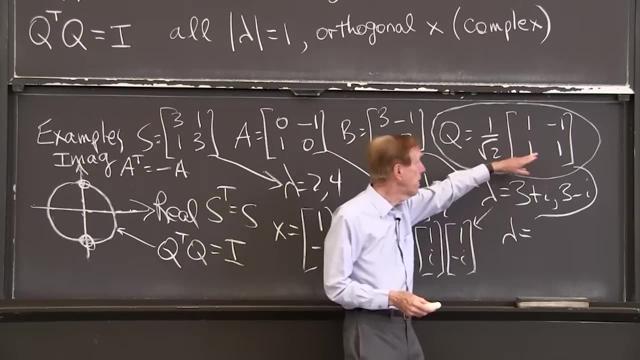 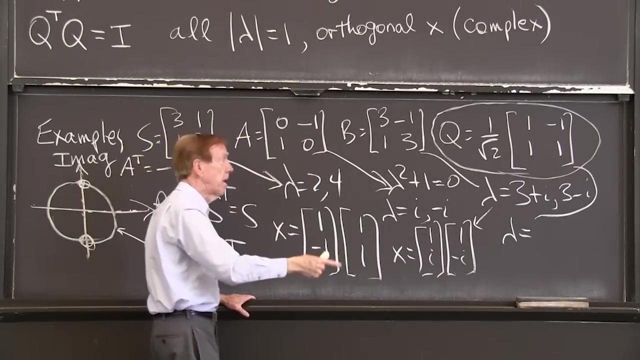 And finally this one, the orthogonal matrix. what are the eigenvalues of that? Let's see. I can see here I've added 1 times the identity, just added the identity to minus 1, 1.. So again I have this minus 1, 1 plus the identity. 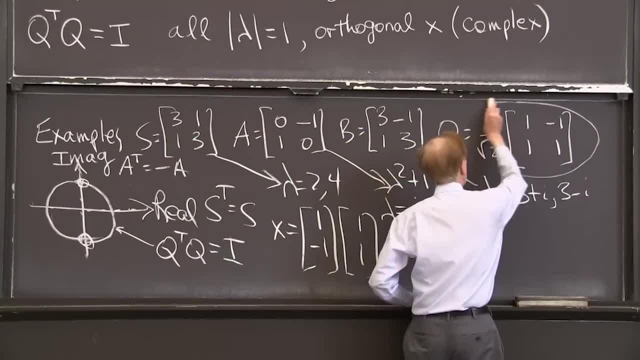 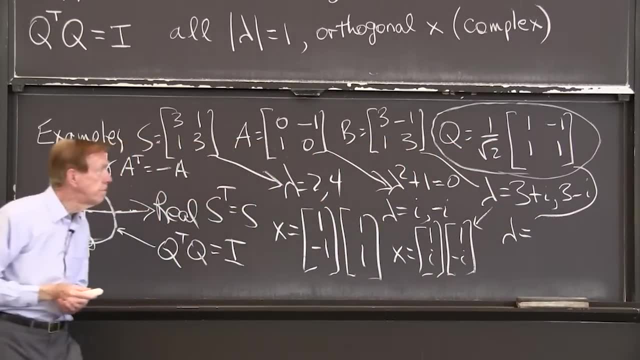 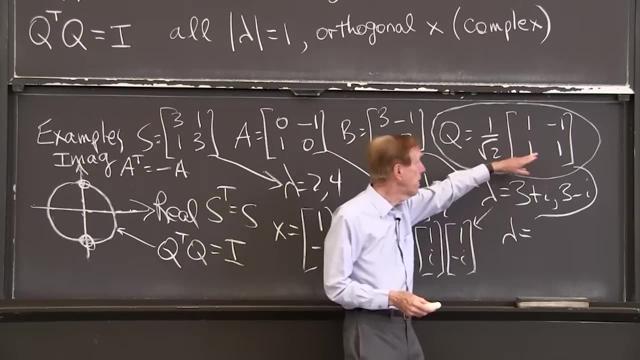 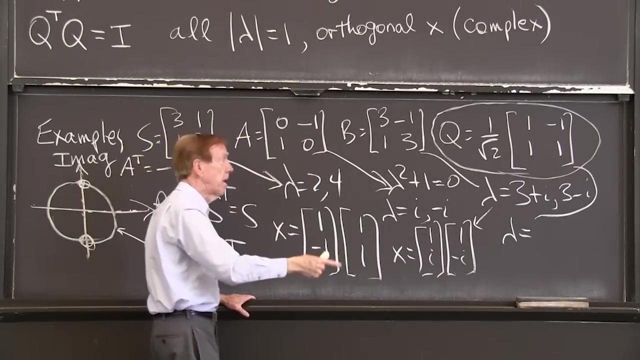 And finally this one, the orthogonal matrix. what are the eigenvalues of that? Let's see. I can see here I've added 1 times the identity, just added the identity to minus 1, 1.. So again I have this minus 1, 1 plus the identity. 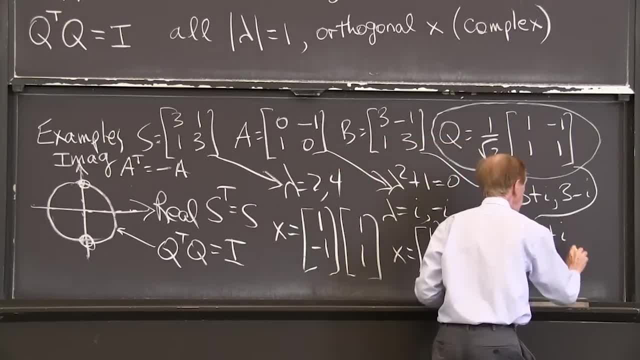 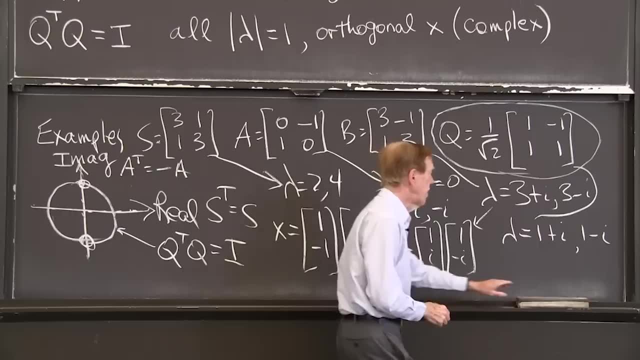 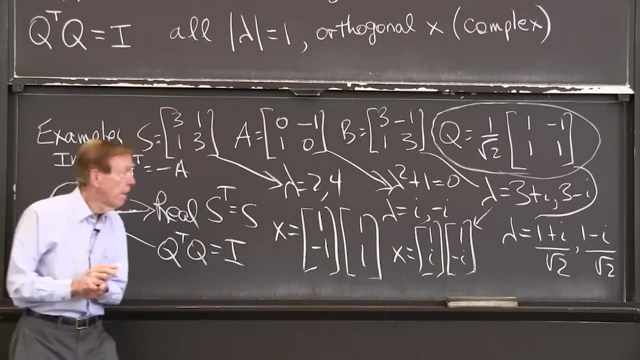 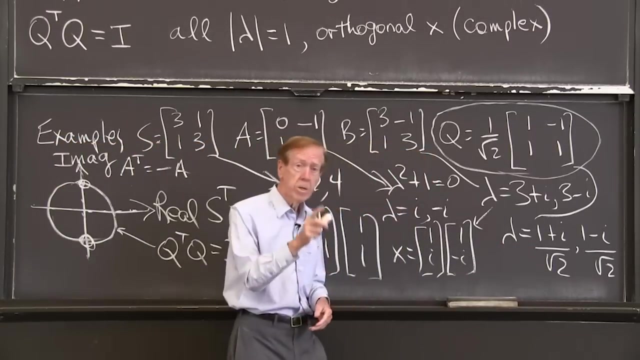 So I would have 1 plus i and 1 minus i from the matrix And now I've got a difference Division by square root of 2, square root of 2. And those numbers lambda. you recognize that when you see that number that is on the unit circle. 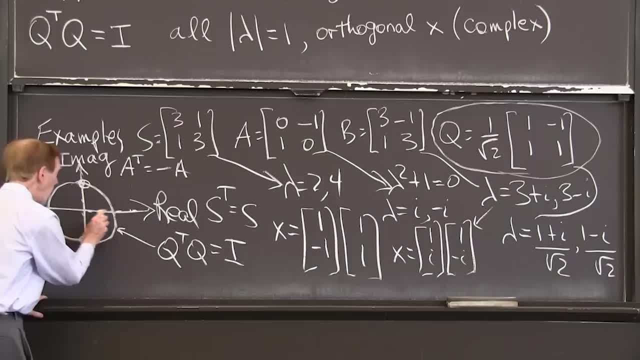 Where is it? on the unit circle 1 plus i, 1 plus i over square root of 2.. Square root of 2 brings it down there. There's 1.. There's, i Divide by square root of 2.. 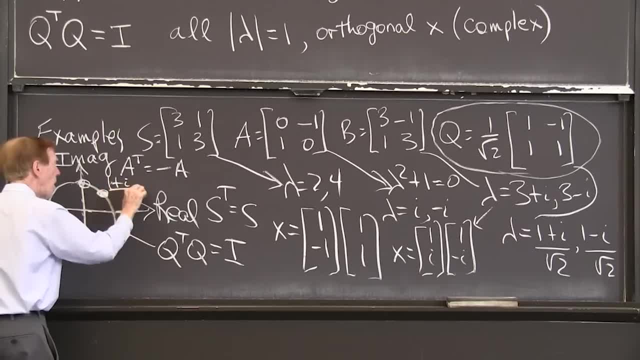 That puts us on the unit circle. That puts us on the circle That's 1 plus i over square root of 2. And here's 1 plus i, 1 minus i over square root of 2. Complex conjugates that number. when I say complex conjugate, 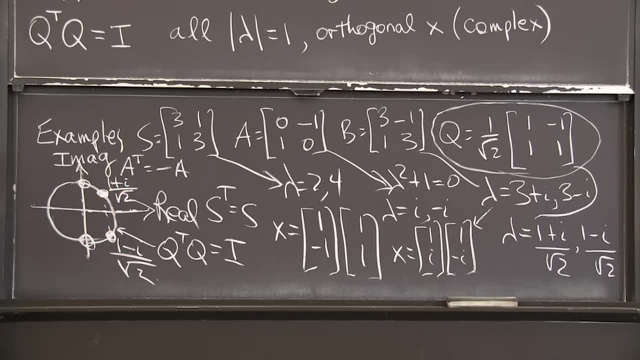 that means I change every i to a minus i, I go, I flip across the real axis. I want to do that in a minute. So are there more lessons to see for these examples? Again, real eigenvalues and real eigenvectors, no problem. 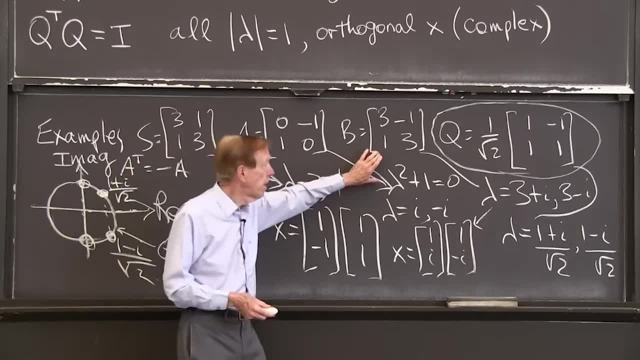 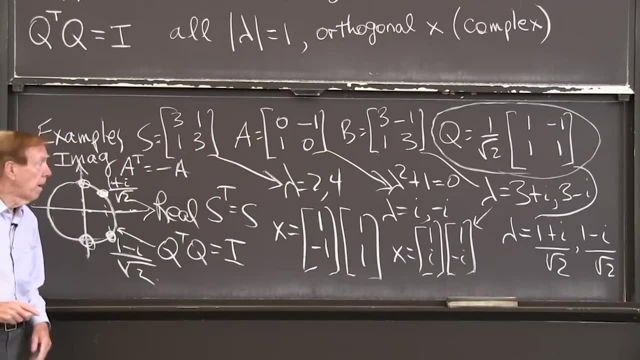 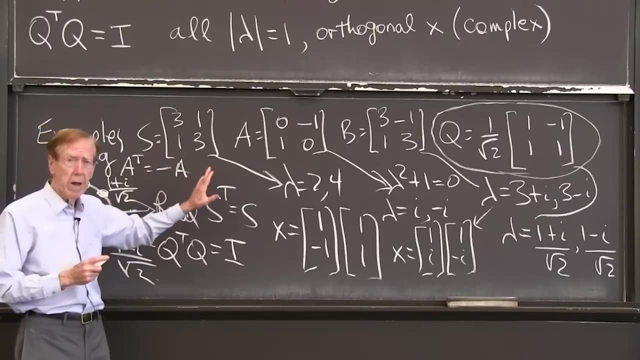 Here imaginary eigenvalues Here complex eigenvalues Here complex eigenvalues on the circle, On the circle. OK, And each of those facts that I just said about the location of the eigenvalues has a short proof, but maybe I'll. 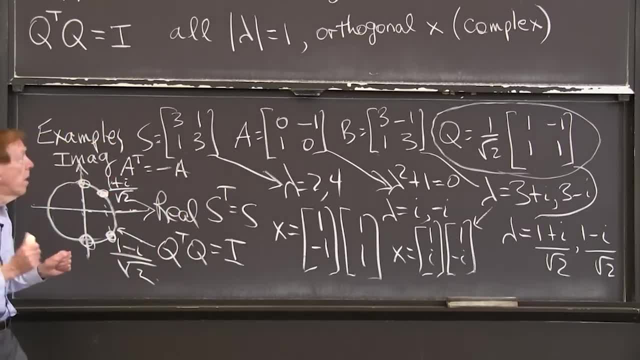 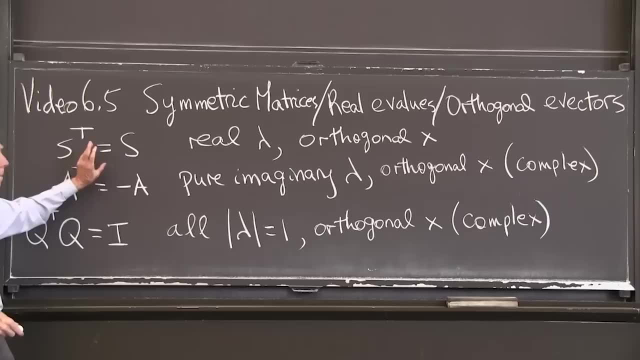 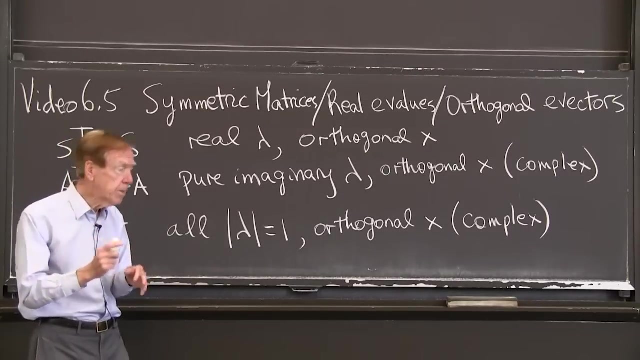 Won't give the proof here, It's the fact that you want to remember. Can I bring down again just for a moment these main facts: Real from symmetric, imaginary from anti-symmetric. magnitude 1 from orthogonal. OK, Now I feel I'm talking about complex numbers. 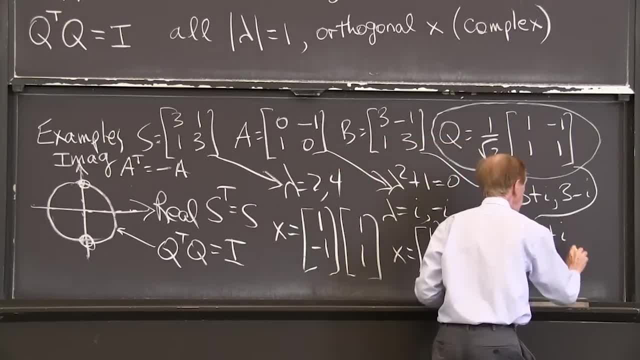 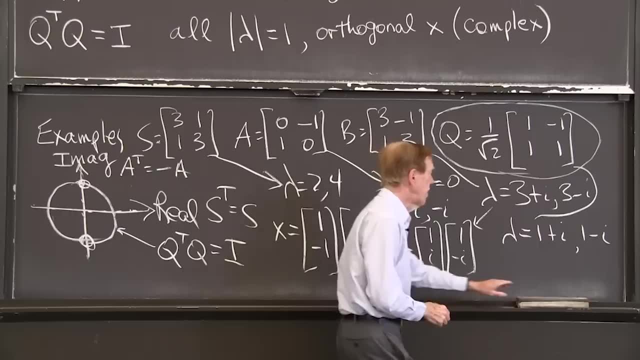 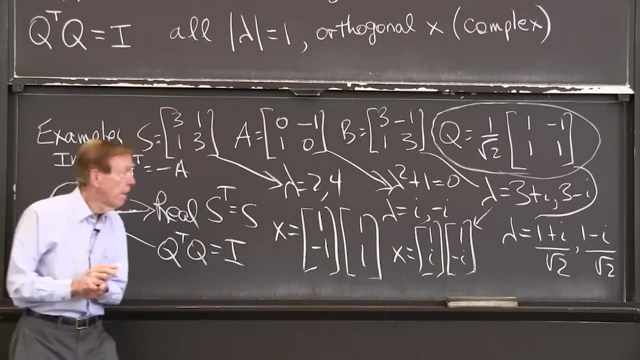 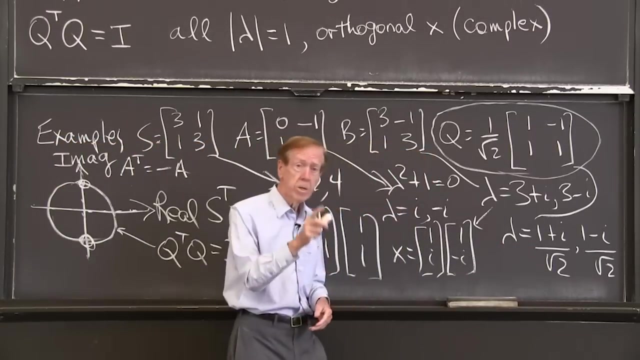 So I would have 1 plus i and 1 minus i from the matrix And now I've got a difference Division by square root of 2, square root of 2. And those numbers lambda. you recognize that when you see that number that is on the unit circle. 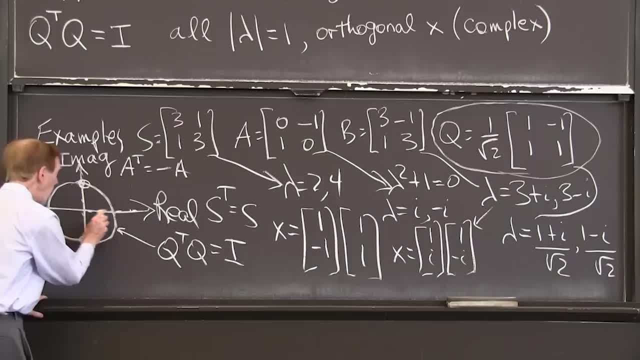 Where is it? on the unit circle 1 plus i, 1 plus i over square root of 2.. Square root of 2 brings it down there. There's 1.. There's, i Divide by square root of 2.. 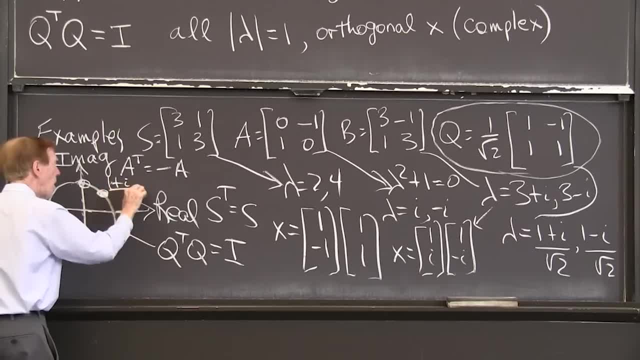 That puts us on there, On the circle. that's 1 plus i over square root of 2. And here's 1 plus i, 1 minus i over square root of 2.. Complex conjugates: That number when I say complex conjugate. 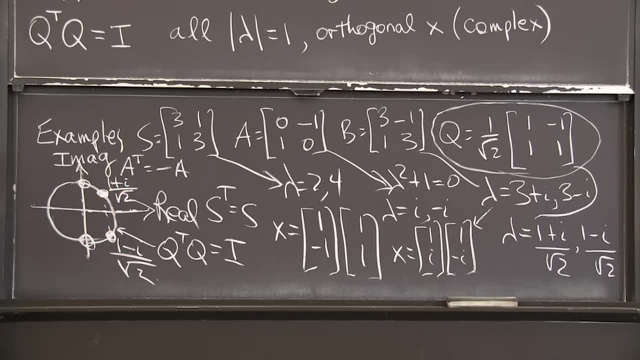 that means I change every i to a minus i. I flip across the real axis. I want to do that in a minute. So are there more lessons to see for these examples? Again, real eigenvalues and real eigenvectors, no problem. 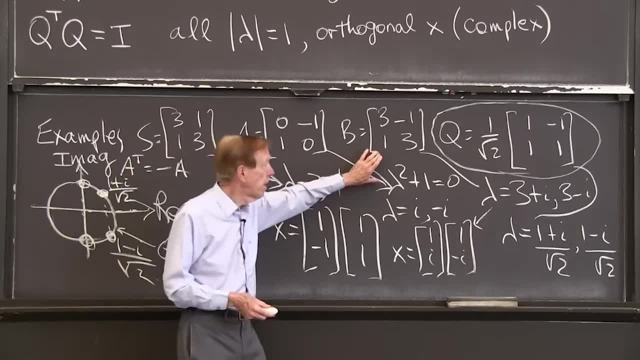 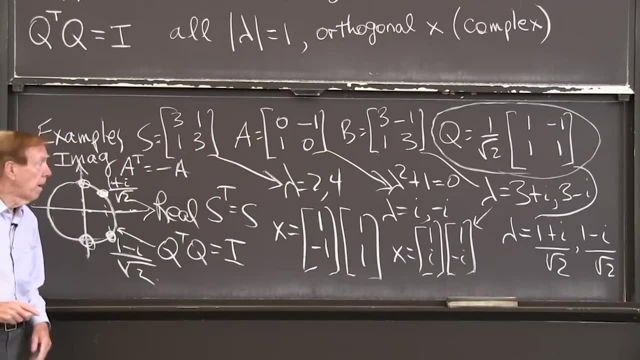 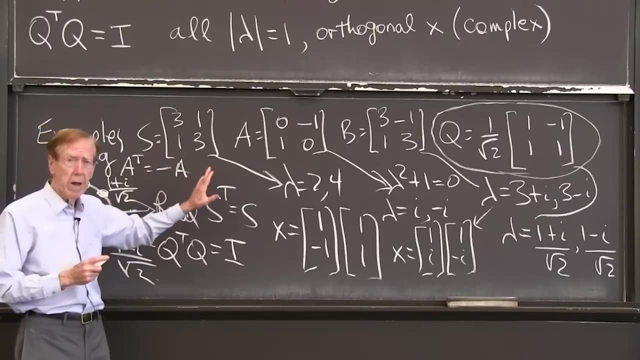 Here imaginary eigenvalues Here complex eigenvalues Here complex eigenvalues on the circle, On the circle. OK, And each of those facts that I just said about the location of the eigenvalues has a short proof, but maybe I'll. 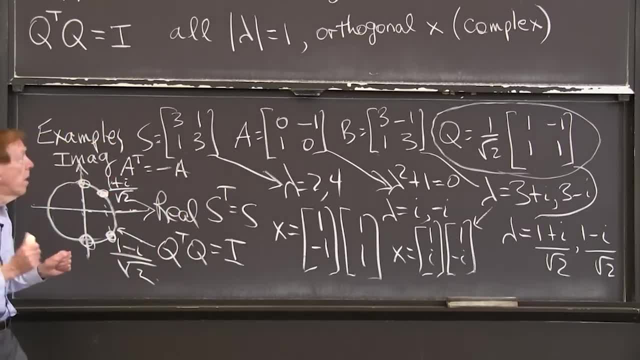 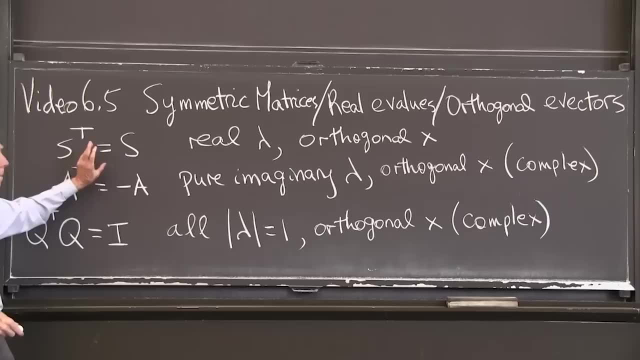 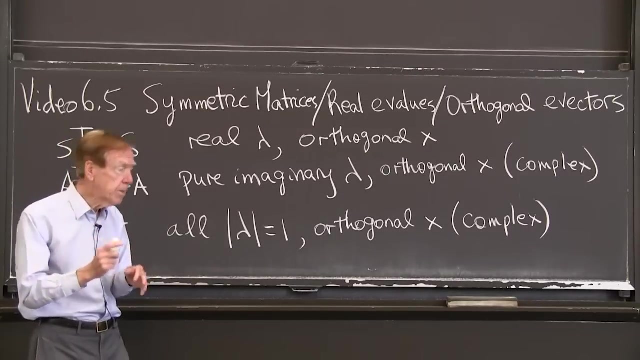 Won't give the proof here, It's the fact that you want to remember. Can I bring down again just for a moment these main facts: Real from symmetric, imaginary from anti-symmetric. magnitude 1 from orthogonal. OK, Now I feel I'm talking about complex numbers. 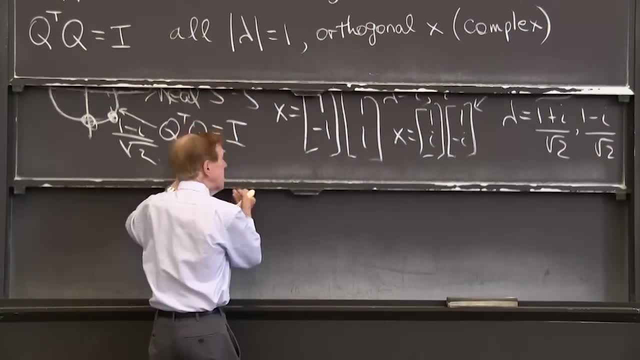 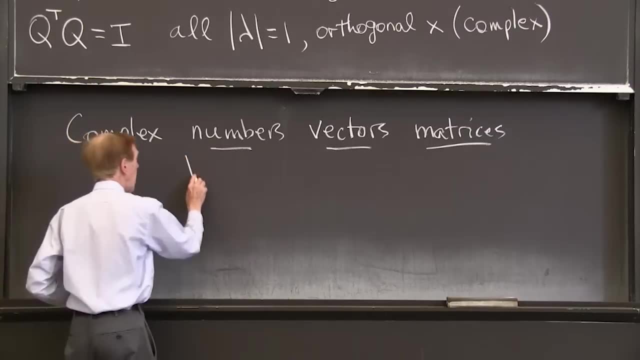 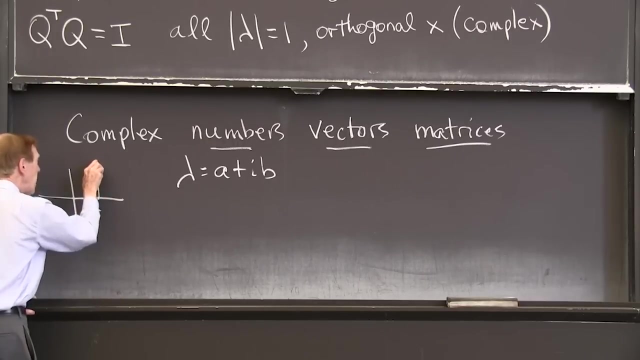 and I really should say I should pay attention to that. Complex numbers. So I have lambda is a plus ib. What do I mean by the magnitude of that number? What's the magnitude of lambda is a plus ib? Again, I go along a up b. 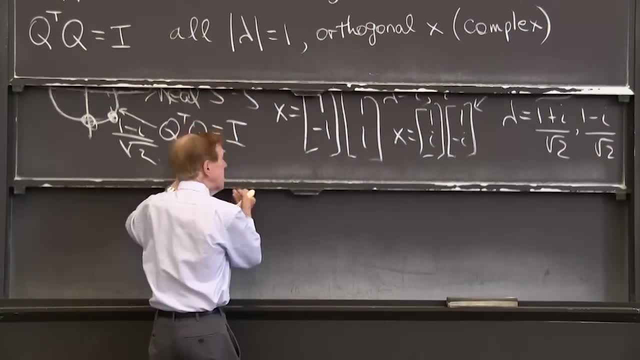 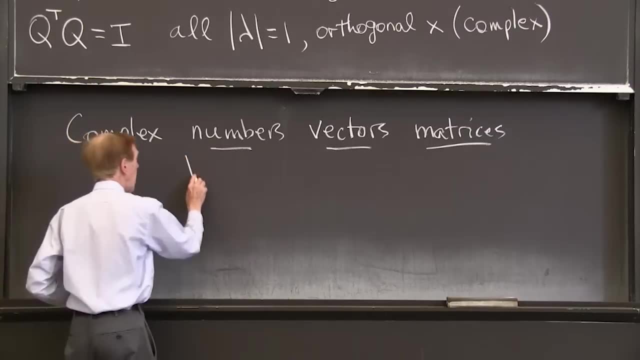 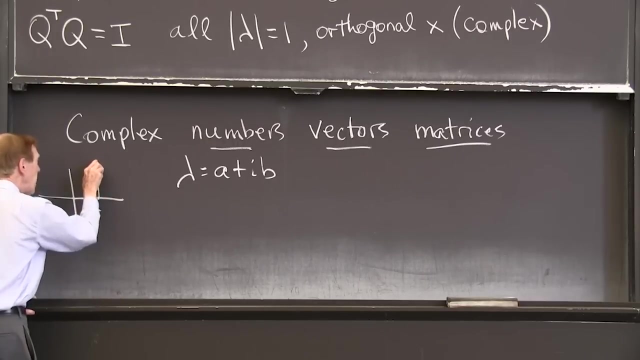 and I really should say I should pay attention to that. Complex numbers. So I have lambda is a plus ib. What do I mean by the magnitude of that number? What's the magnitude of lambda is a plus ib? Again, I go along a up b. 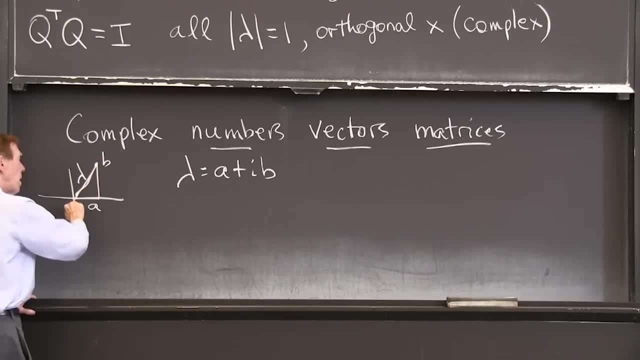 Here is the lambda, The complex number, And I want to know the length of that. Well, everybody knows the length of that. Thank goodness Pythagoras lived, or his team lived. It's the square root of a squared plus b squared. 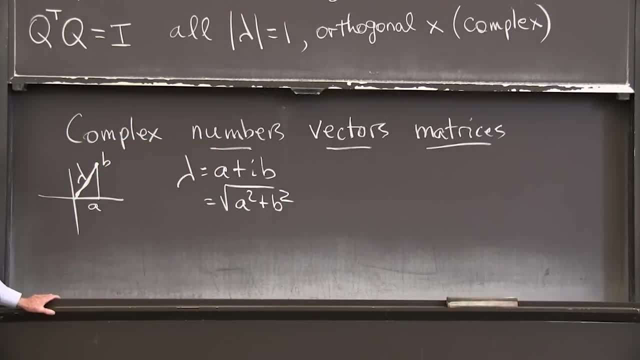 And notice, how do I get that number from this one, This one, It's important: If I multiply a plus ib times a minus ib, So I have lambda, That's a plus ib times lambda, conjugate, That's a minus ib. 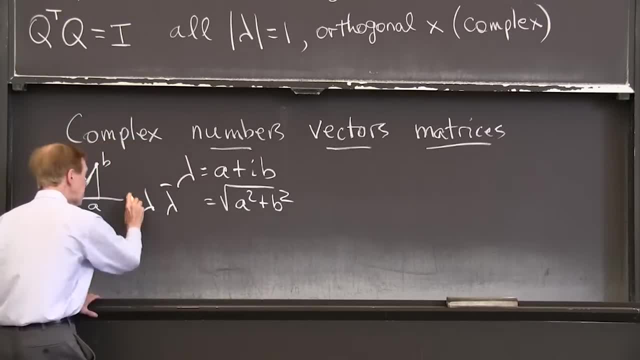 If I multiply those, that gives me a squared plus b squared. So I take the square root And this is what I would call the magnitude of lambda. So the magnitude of a number Is that positive length And it can be found. 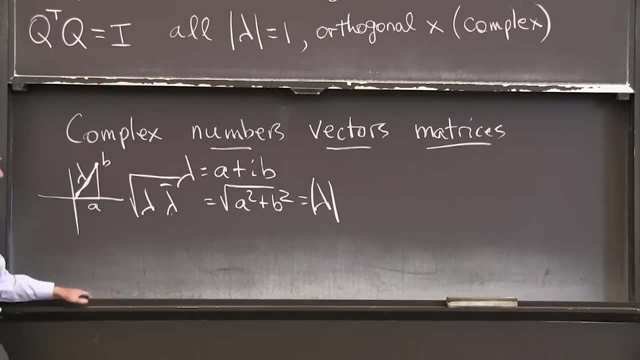 You take the complex number times its conjugate. That gives you a squared plus b squared, And then take the square root. Basic facts about complex numbers. OK, what about complex vectors? What is the dot product? What is the correct? x transpose x. 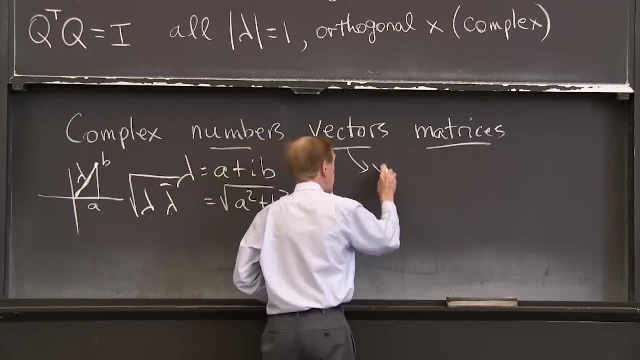 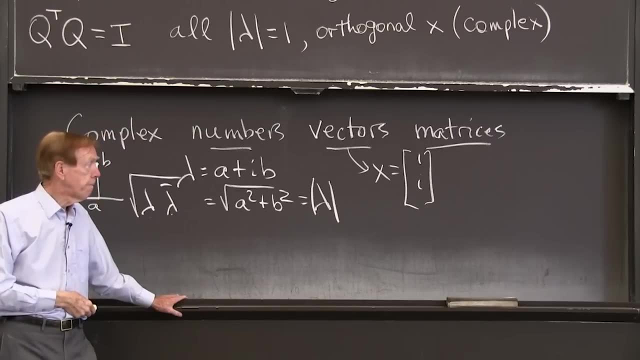 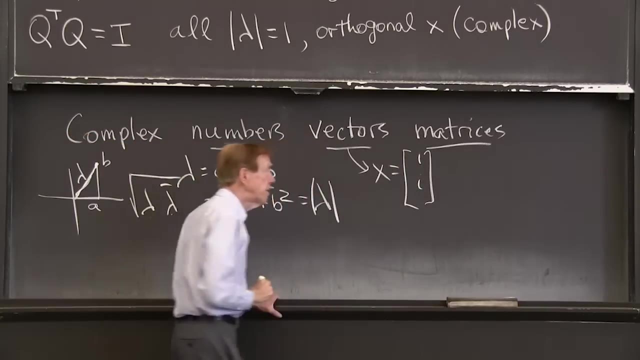 Well, it's not x. transpose x. Suppose x is the vector 1.. 1i, As we saw that as an eigenvector. What's the length of that vector? The length of that vector is not 1 squared plus i squared. 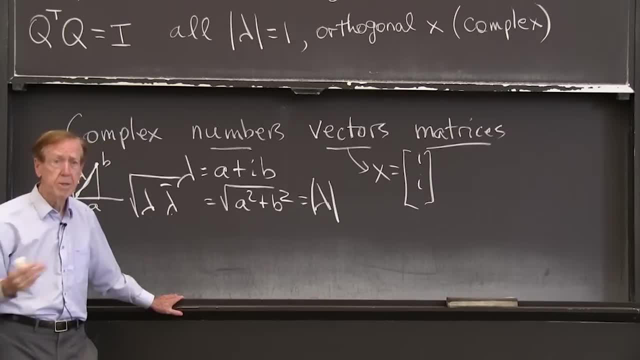 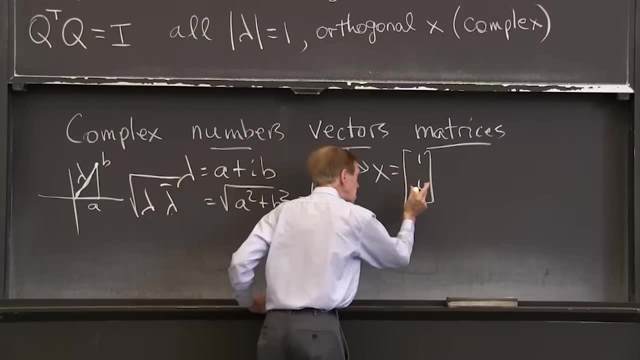 1 squared plus i squared would be 1 plus minus 1 would be 0.. The length of that vector is the size of this squared plus the size of this squared square root. So the length, Here we go. The length of x squared. 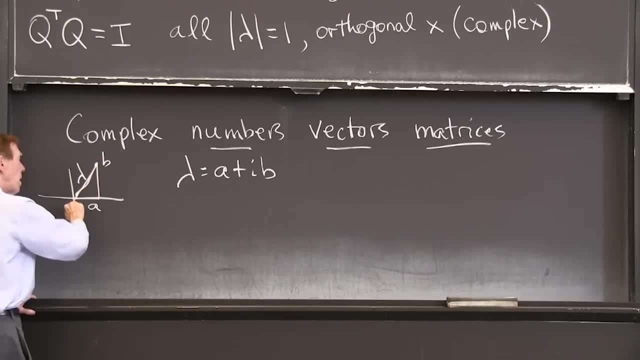 Here is the lambda, The complex number, And I want to know the length of that. Well, everybody knows the length of that. Thank goodness Pythagoras lived, or his team lived. It's the square root of a squared plus b squared. 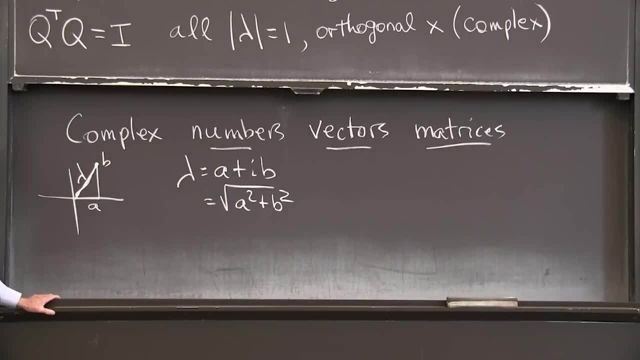 And notice, how do I get that number from this one, This one, It's important: If I multiply a plus ib times a minus ib, So I have lambda, That's a plus ib times lambda, conjugate, That's a minus ib. 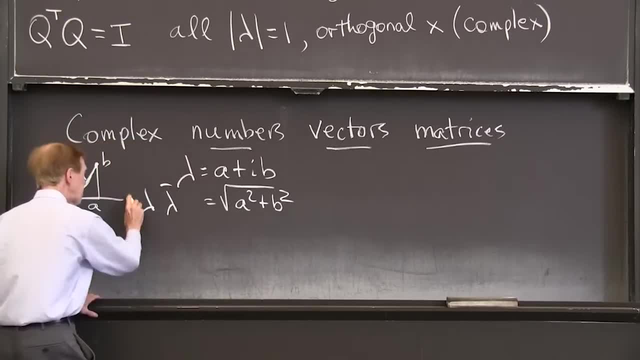 If I multiply those, that gives me a squared plus b squared. So I take the square root And this is what I would call the magnitude of lambda. So the magnitude of a number Is that positive length And it can be found. 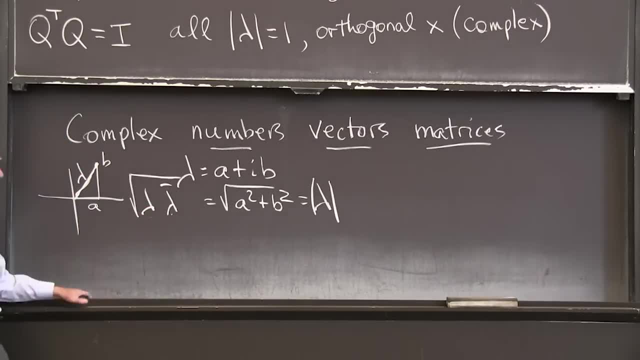 You take the complex number times its conjugate. That gives you a squared plus b squared, And then take the square root. Basic facts about complex numbers. OK, What about complex vectors? What is the dot product? What is the correct? x transpose x. 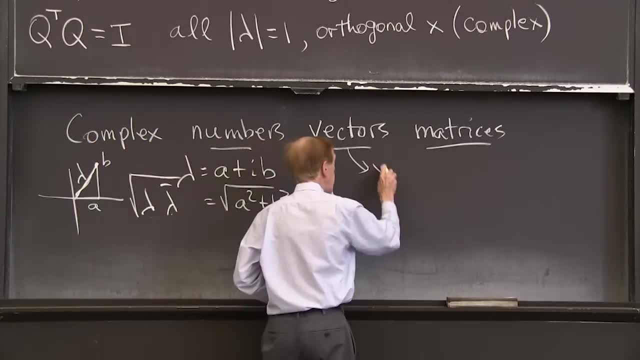 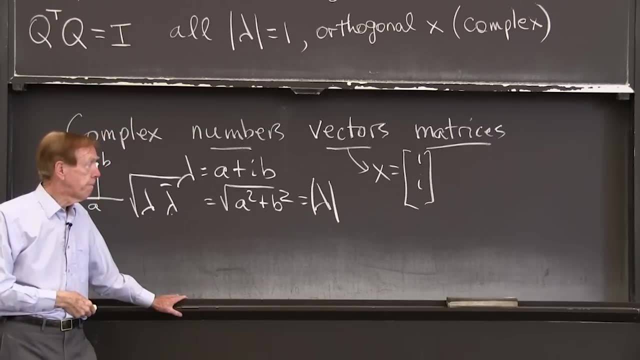 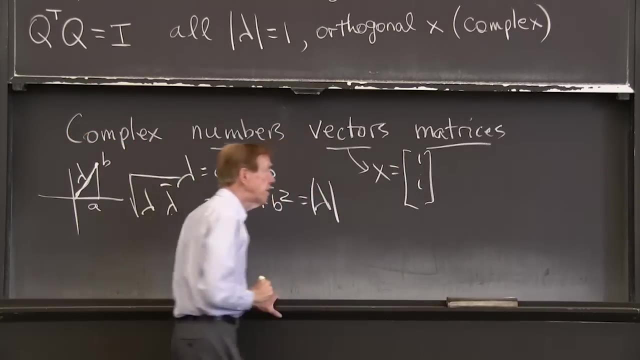 Well, it's not x. transpose x. Suppose x is the vector 1.. I, As we, saw that as an eigenvector. What's the length of that vector? The length of that vector is not 1 squared plus i squared. 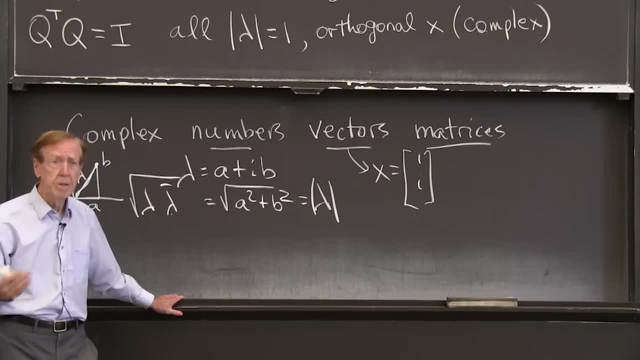 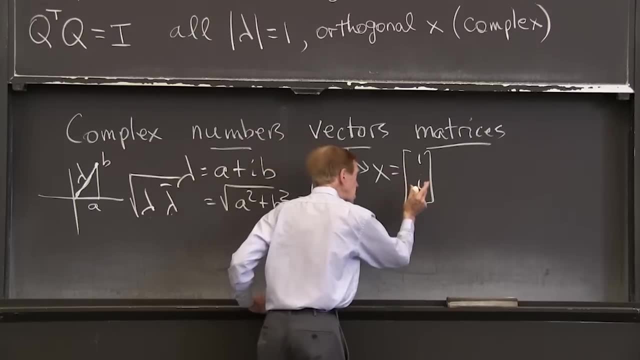 1 squared plus i squared would be 1 plus minus 1 would be 0.. The length of that vector is the size of this squared plus the size of this squared square root. So the length, Here we go. The length of x. 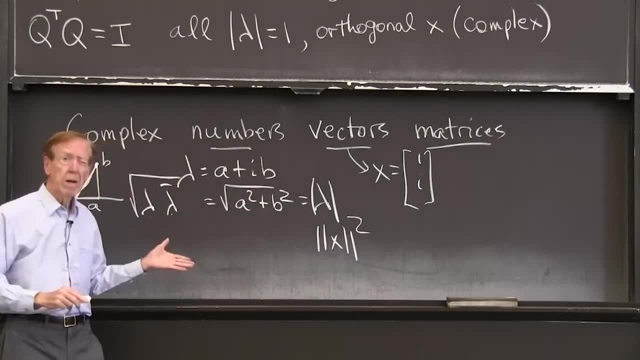 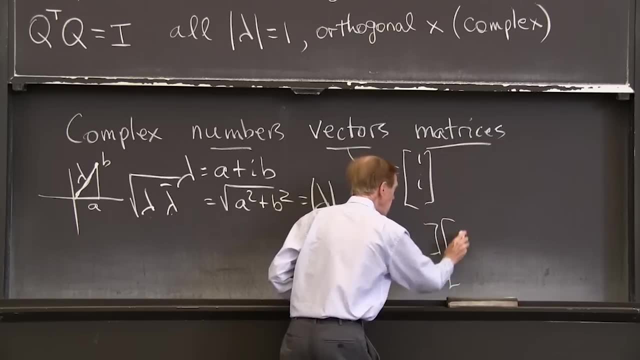 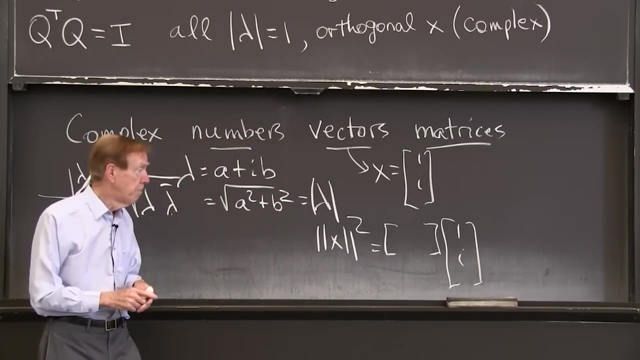 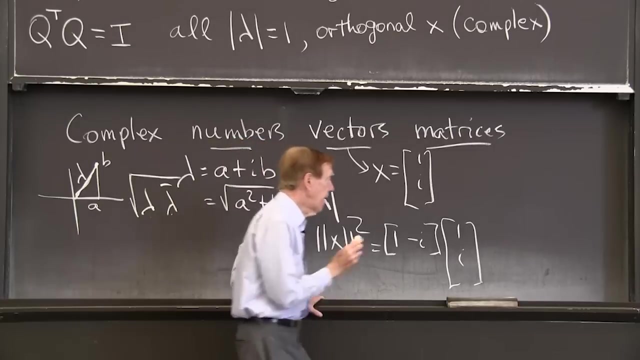 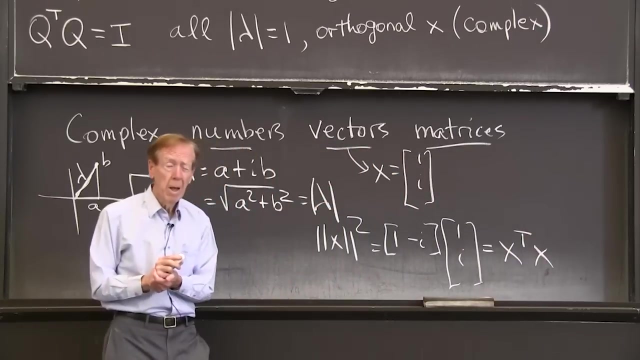 Of x squared, The length of the vector squared will be the vector. As always. I can find it from a dot product, But I have to take the conjugate of that. If I want the length of x, I would usually take x. transpose x right. 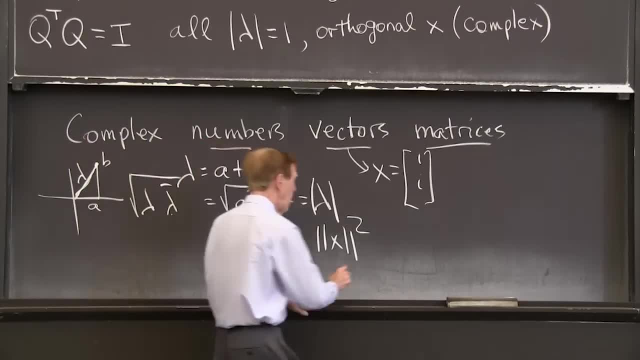 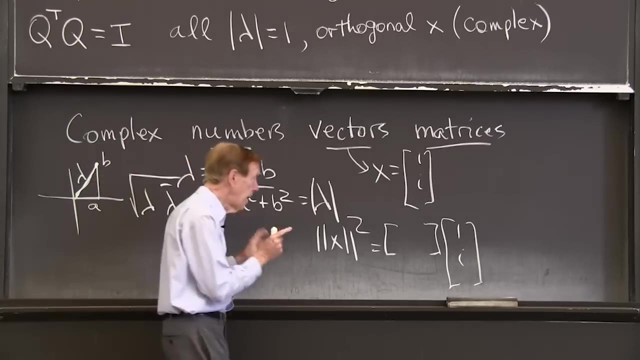 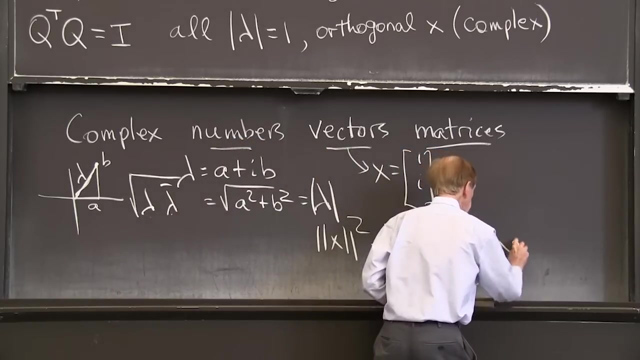 The length of the vector squared will be the vector. As always, I can find it from a dot product, But I have to take the conjugate of that. If I want the length of x I have to take usually take x, transpose x, right. 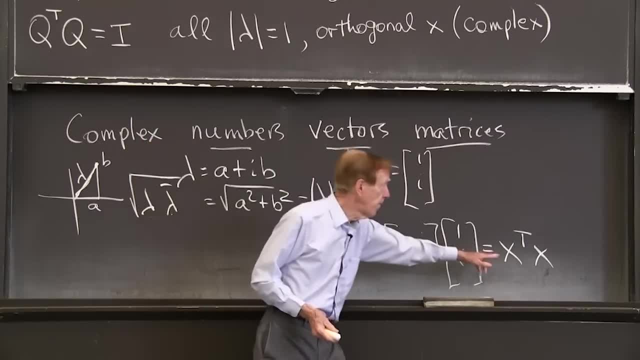 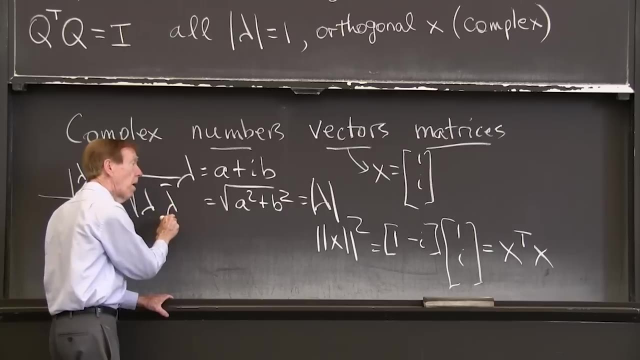 If I have a real vector x, then I find its dot product with itself And Pythagoras tells me I have the length squared. But if the things are complex, I want minus, i times i. I want to get lambda times, lambda bar. 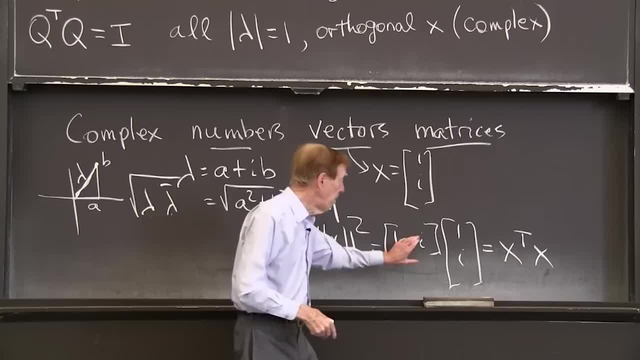 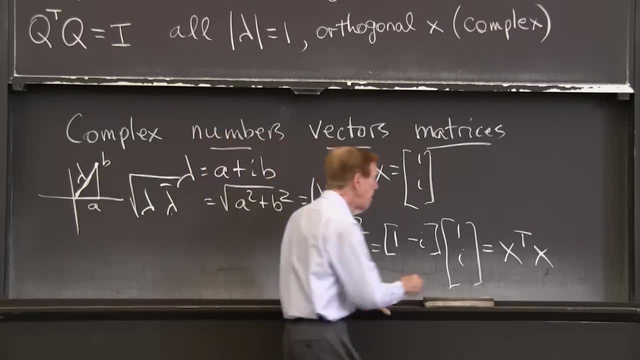 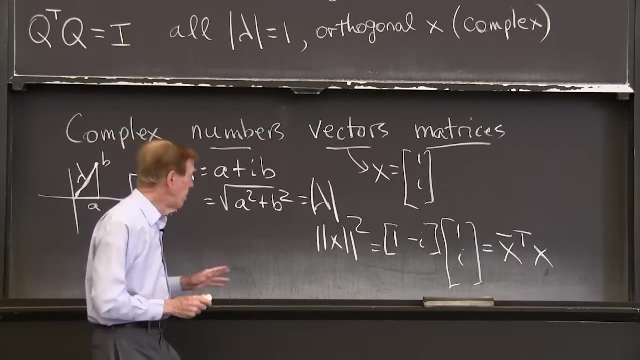 I want to get a positive number. Minus i times i is plus 1.. Minus i times i is plus 1.. So I must, must do that. So that's really what orthogonal would mean: Orthogonal vectors, orthogonal complex vectors. 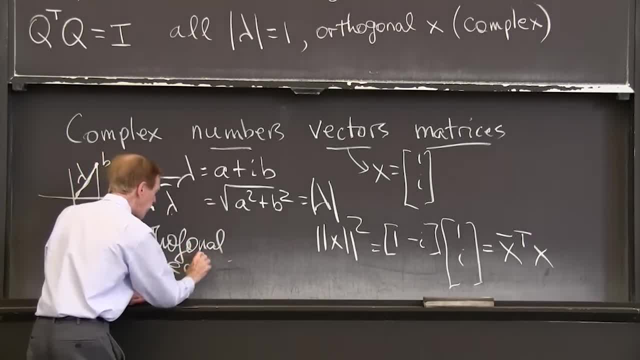 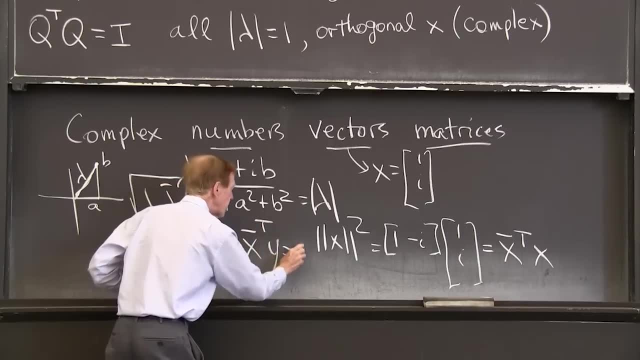 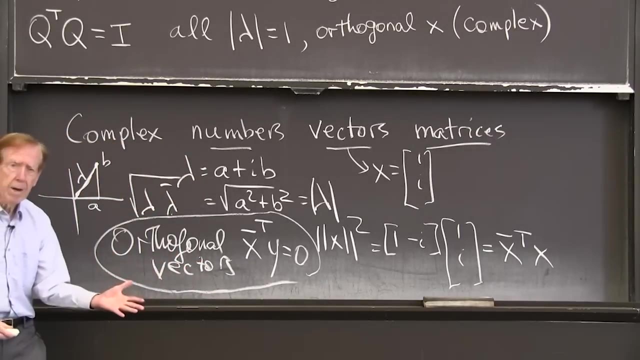 mean orthogonal vectors mean that x conjugate transpose y is 0. That's it. That's what I mean by orthogonal eigenvectors. when those eigenvectors are complex, I must remember to take the complex conjugate, And I also do it for matrices. 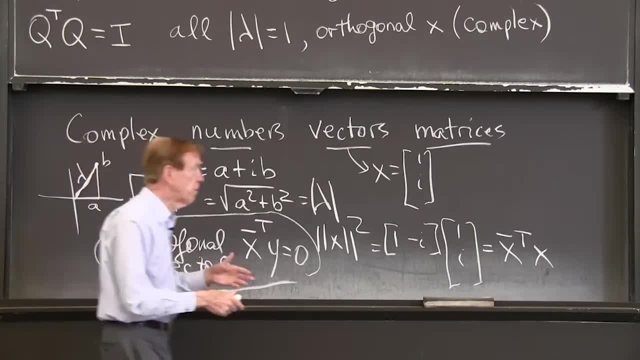 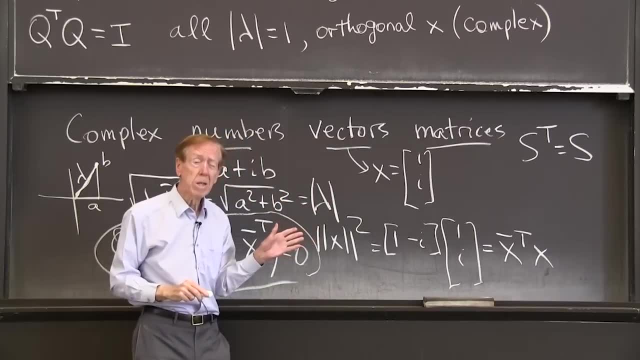 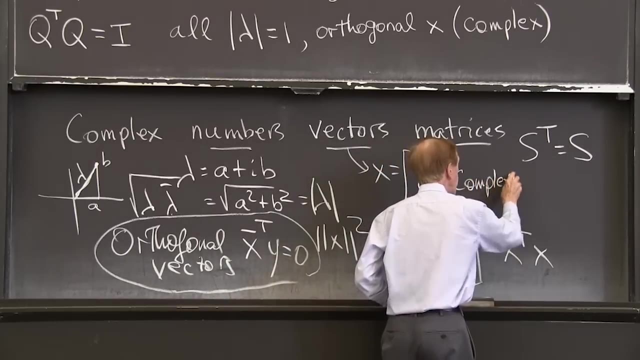 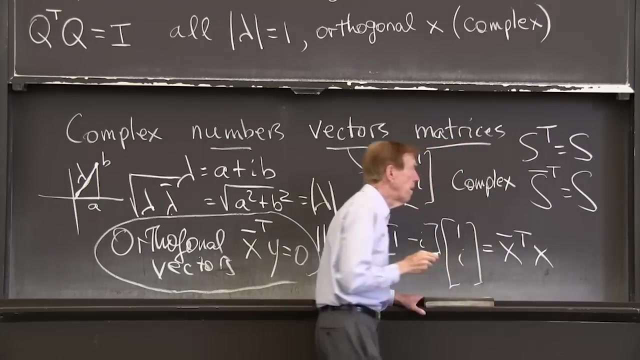 So if I have a symmetric matrix, s transpose s. I know what that means. But suppose s is complex? Suppose s is complex, Then for a complex matrix I would look at s. bar transpose equals s. That's the. that's every time I transpose. 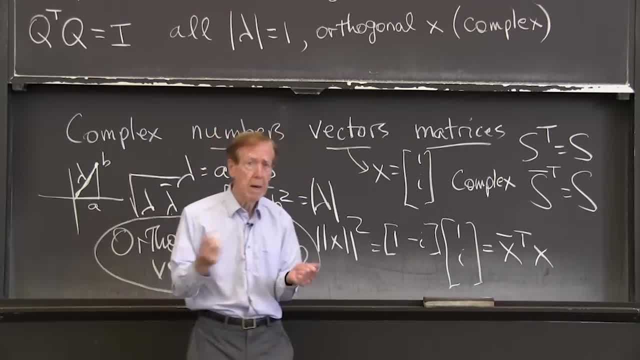 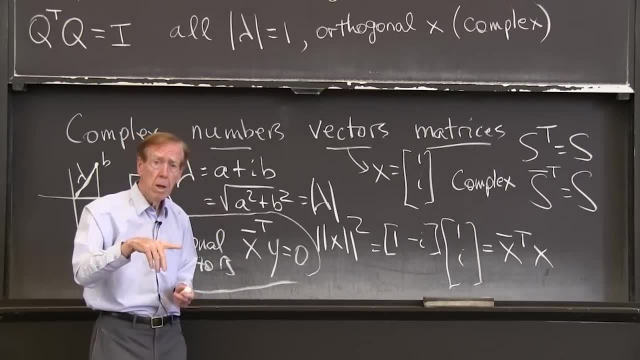 if I have complex numbers, I should take the complex conjugate. MATLAB does that automatically. If you asked for x prime, it will produce, not just it'll change a column to a row with that, transpose that prime And It. 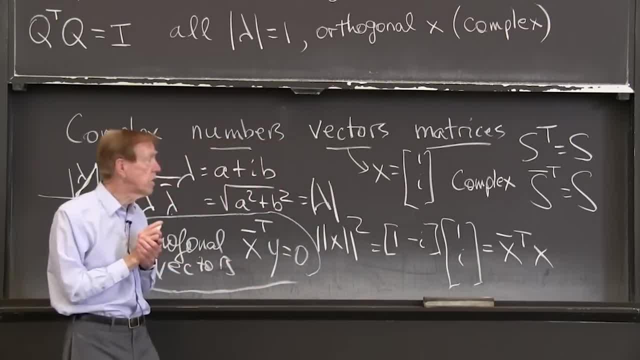 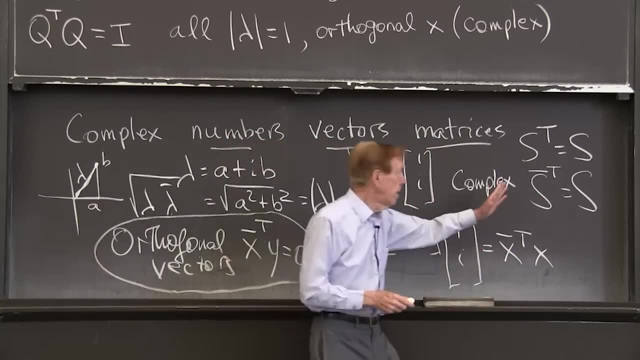 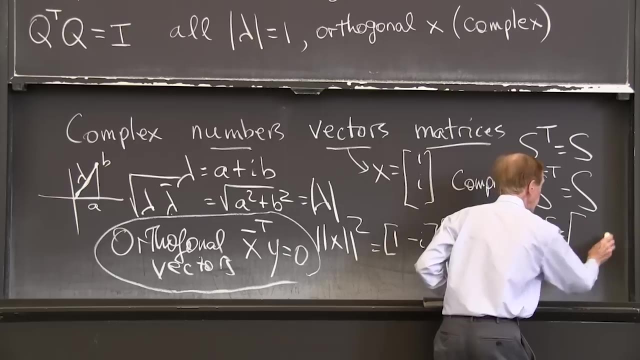 Takes a complex conjugate. So we must remember always to do that. Yeah, And in fact if s was a complex matrix, but it had that property, let me give an example. So here's an s an example of that. 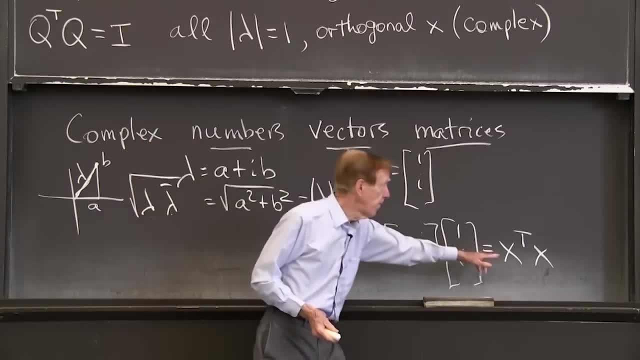 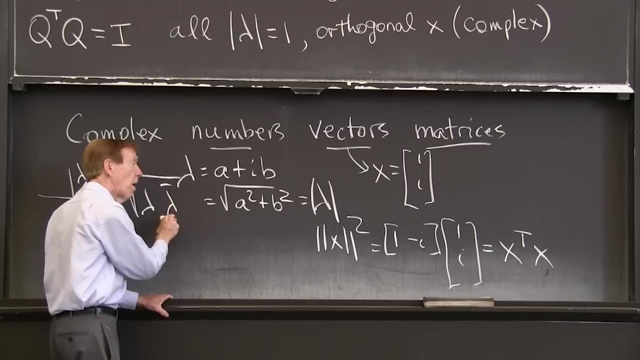 If I have a real vector x, then I find its dot product with itself And Pythagoras tells me I have the length squared. But if the things are complex, I want minus, i times i. I want to get lambda times, lambda bar. 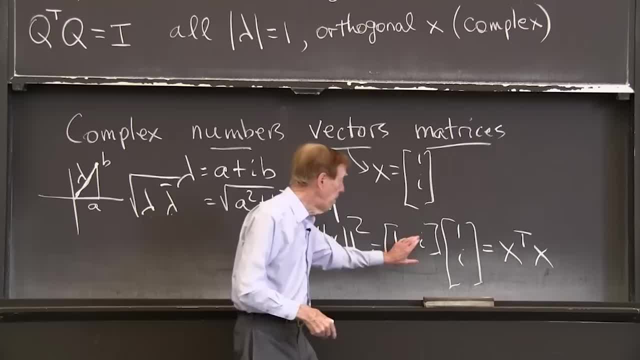 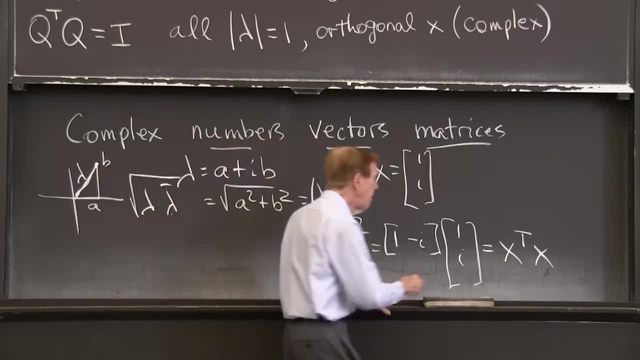 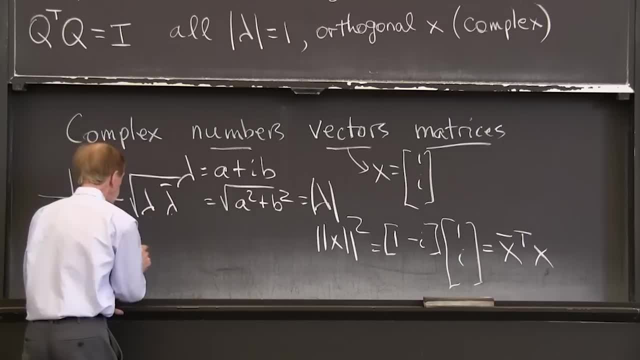 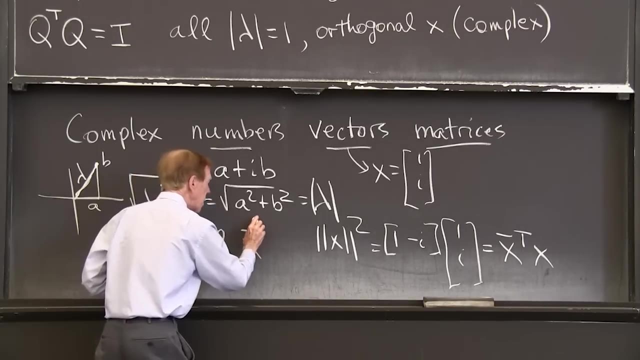 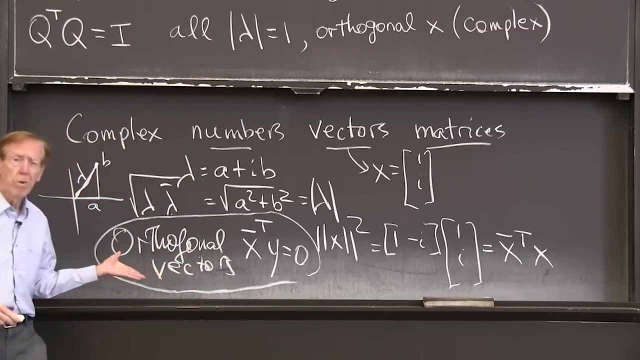 So that's really what orthogonal would mean. Orthogonal vectors, orthogonal complex vectors mean. orthogonal vectors mean that x conjure, transpose, y is 0. That's what I'm going to do. That's what I'm going to do. That's what I mean by orthogonal eigenvectors. 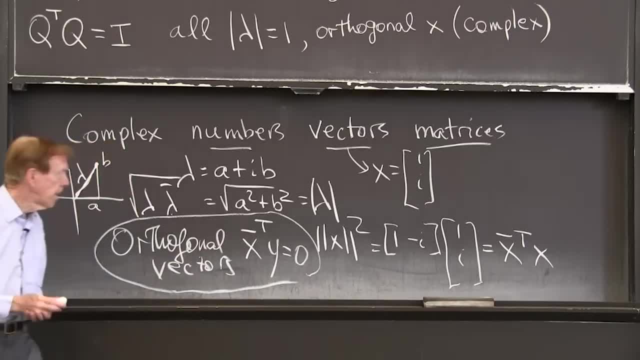 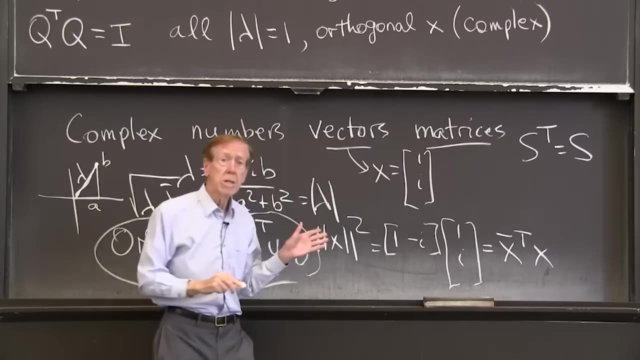 when those eigenvectors are complex. I must remember to take the complex conjugate, And I also do it for matrices. So if I have a symmetric matrix s transpose s, I know what that means. But suppose s is complex. Suppose s is complex. 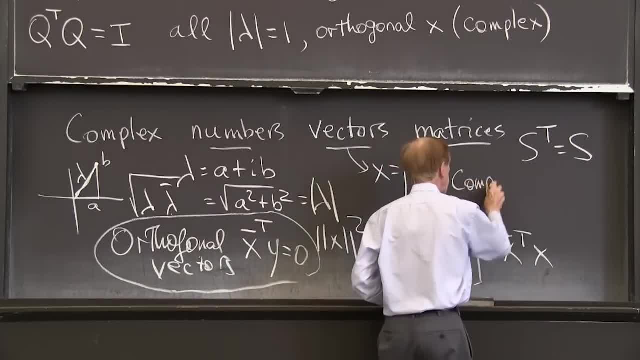 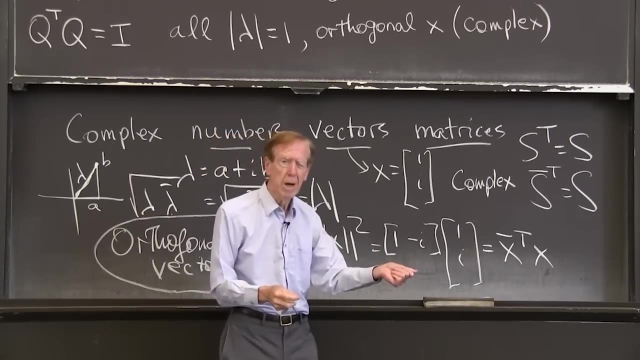 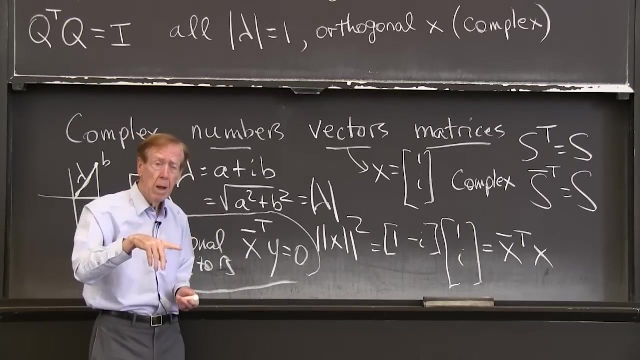 Then for complex matrix I would look at s. Look at s. bar transpose equals s. That's the. that's every time I transpose. if I have complex numbers, I should take the complex conjugate MATLAB. does that automatically. If you asked for x prime, it will produce, not just. 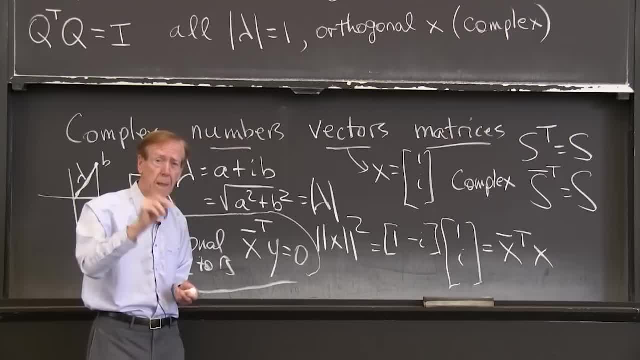 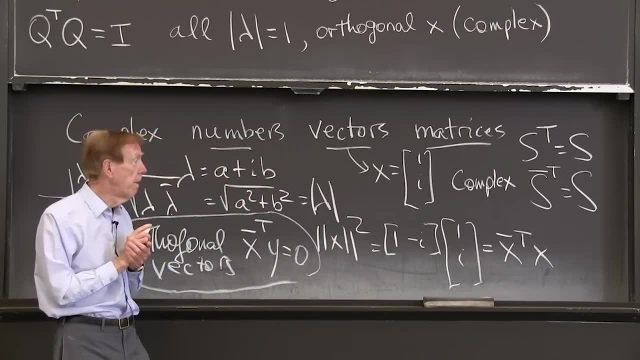 it'll change a column to a row with that: transpose that prime And it will take the complex conjugate. It will take the complex conjugate, So we must remember always to do that. Yeah, And in fact if s was a complex matrix. 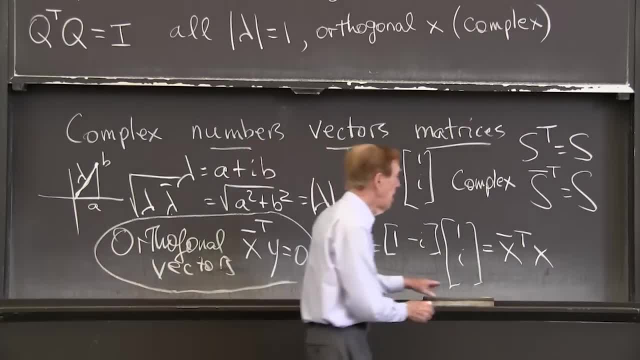 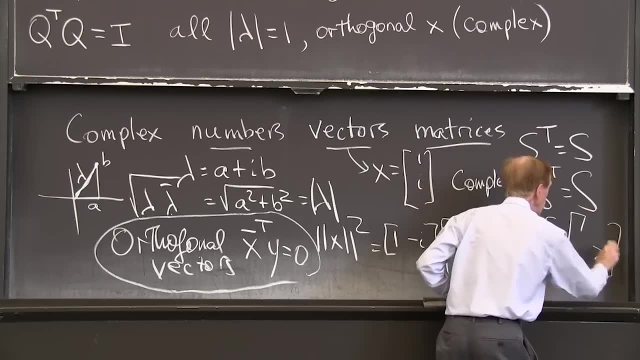 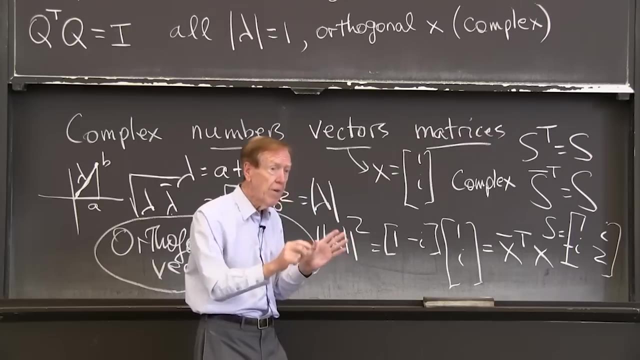 but it had that property. let me give an example. So here's an s an example of that 1, 2, i and minus i. So I have a complex matrix And if I transpose it and take complex conjugates,